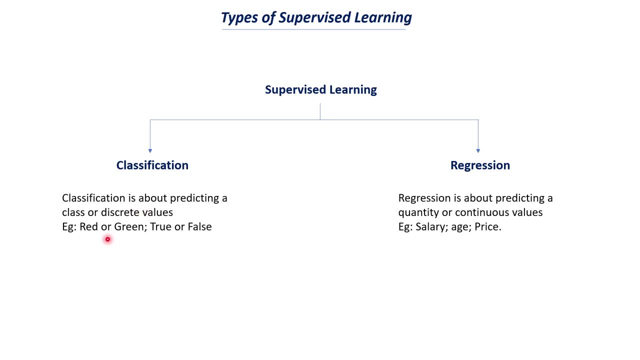 these two. The example of this classification is like predicting whether an object is red in color or green in color, or true or false, whether a person is having diabetes or not. So this is like example of classification problem, whereas predicting the salary of a person or age, or predicting the 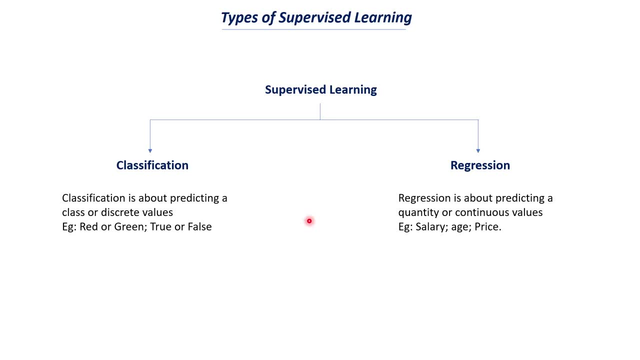 price of a house or a car is a problem. So this is like an example of classification problem, whereas so these comes under regression, ok, And the model evaluation technique for classification problem. So once such example is accuracy score, ok, and in the case of regression we cannot. 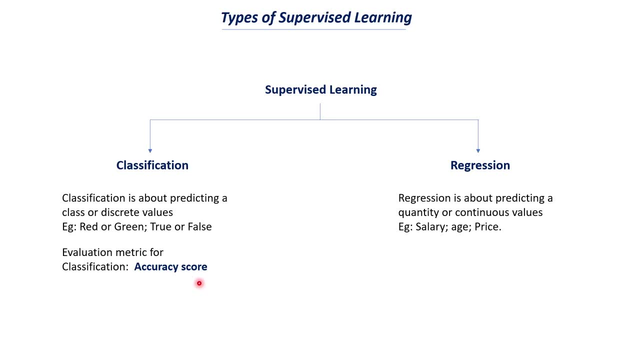 use this accuracy score, So i will explain you why we cant use that- and whereas in the case of regression, we use this error values like mean, absolute error, mean, squared error, etcetera. So we will discuss about this regression evaluation matrix later, But let's try to understand about this. 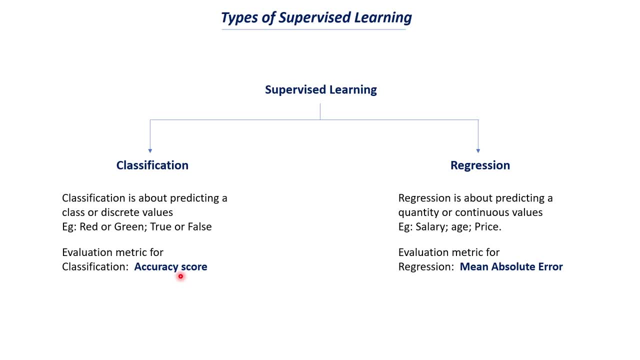 accuracy score. So be, we are calculating this And you know what is the limitation of this accuracy score and why we need this confusion matrix. so these are the things that we will be discussing in this particular video. so i'll just start with the definition of this accuracy. 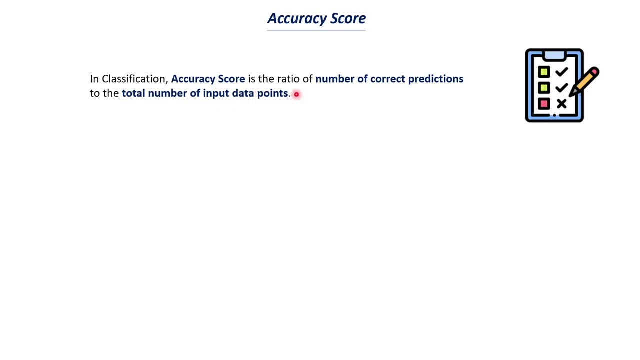 score in classification problems. accuracy score is the ratio of number of correct predictions to the total number of input data points. okay, so what we take here is like we need two values. one is the number of correct predictions made by the model- okay- divided by how many total data points. 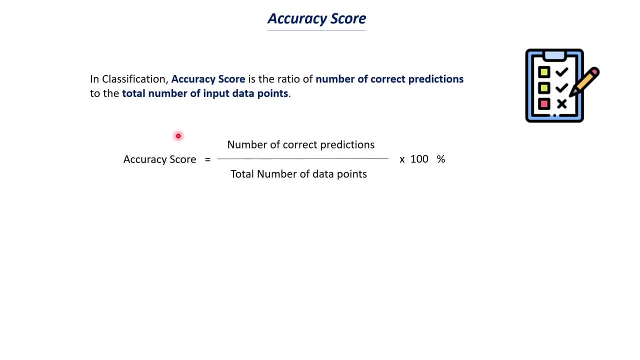 are there for predictions. so let's say that, uh, you know, we can consider the accuracy score formula, something like this accuracy score is equal to we take- we have to take- this number of correct predictions, so we have to divide it by total number of data points, and so this value will be. 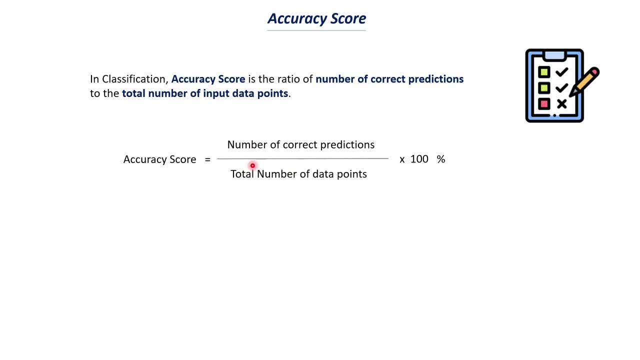 uh, you know between 0 to 1, so like it will be 0.80 or 0.90. so if the accuracy score value is 0.95, that means the model is 95 percent accurate. in order to convert it to a percentage, we can: 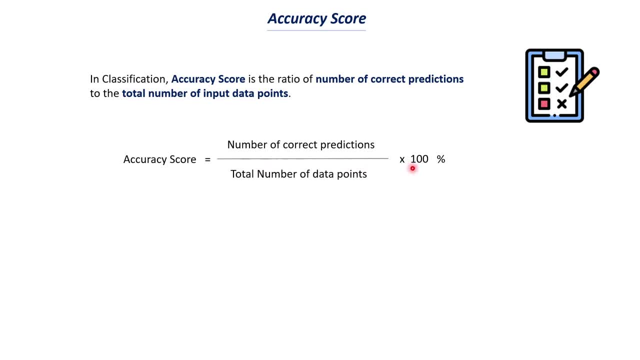 multiply it with android, so it the value will be in percentage. okay, let's try to understand this with an example. let's say that, uh, the number of correct predictions made by the model in a case is 128. okay, let's say that we are building a machine learning. 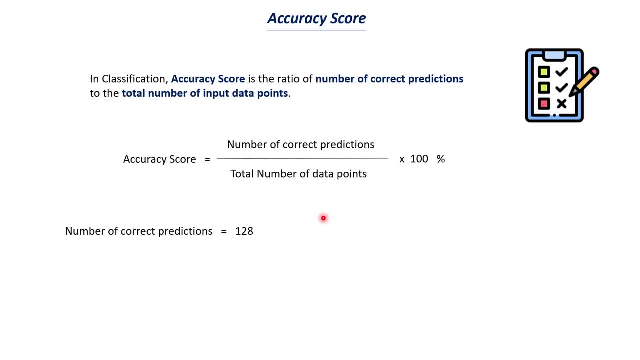 model that can predict whether a person has diabetes or not, and uh, so out of the test data that we are going to predict, the model is making correct predictions for 128 and the total number of data points that we have is 150. okay, so we are taking 150 people based on like some factors like 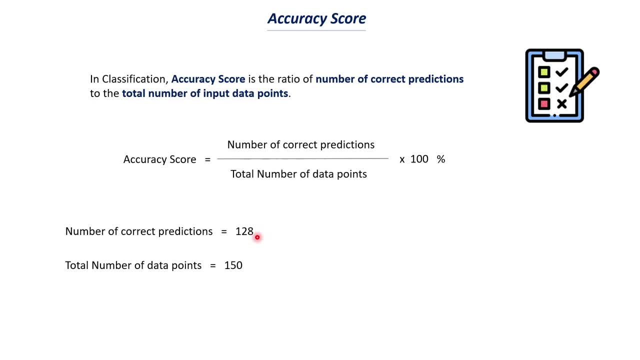 what is their- uh, you know- age, what is their gender and so on, so that let's say that there are like these factors and based on these factors, we have to determine whether that person is diabetic or not. so, uh, we are checking this for 150 data. 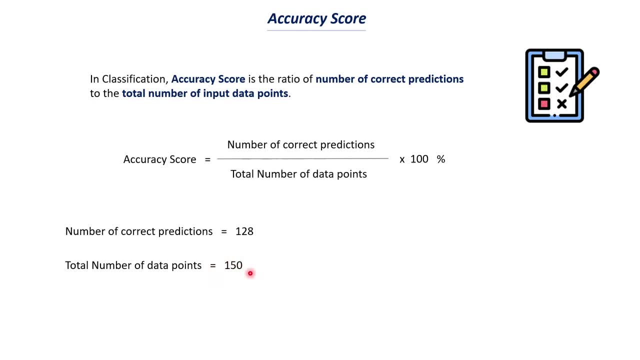 points, or you can consider this as 150 different people. out of this, 150 different people, let's say that the model has predicted correctly for 128 people, or 120 data points, so you just have to plug in these values. so number of correct predictions is 128 and the total number of data points for 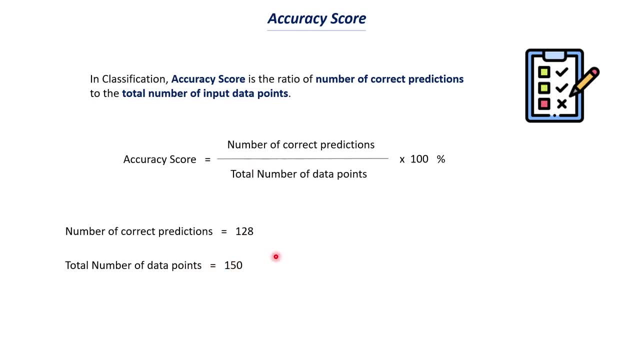 which we are predicting is 150.. so we just have to divide it, and when you divide 128 by 150, this is the value that you get. so 128 by 150 is equal to 0.853, and when you multiply it with 100, you will get 85.3 percentage. so the accuracy score of your model is 85 percentage. what does? 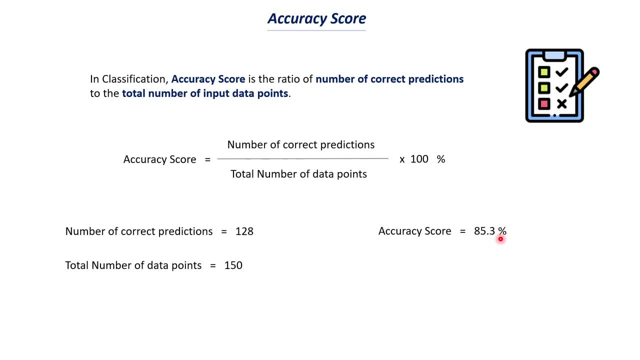 what does this 85 percentage means is, if you uh using this model, if you try to predict uh for under data points, you will get correct predictions for 85 data points. so this is what accuracy score means, generally speaking. so there is not a thumb rule, but we can say that if the accuracy score of 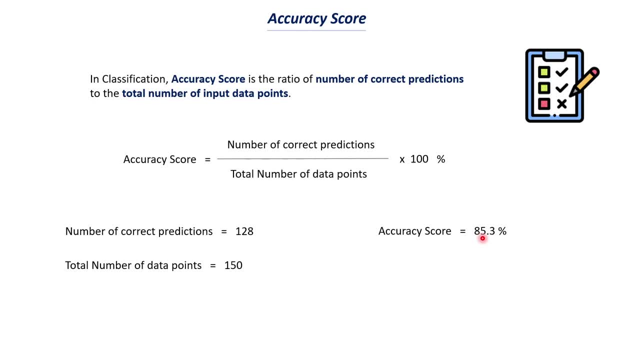 80 percent, then it is like a decent performing model. if the accuracy score is like greater than 90 or 95, then it is like a very good model that can make like accurate predictions. so we can import this accuracy score from this sklein module called as sklein dot matrix. so i'll show you in. 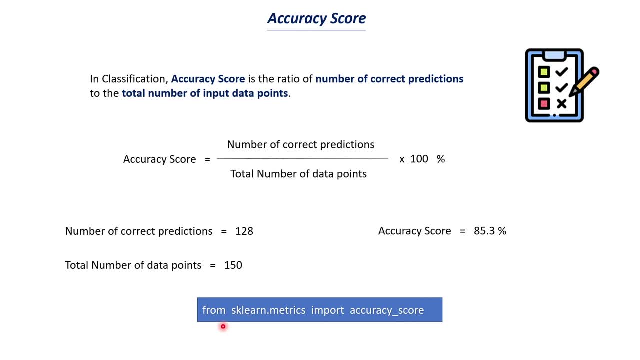 code as well how we can do this. but you can remember that we can import this from from sklein dot matrix import accuracy score and i'm sure that most of you might already know this. so like there is one limitation of this accuracy score. so we have discussed all these. 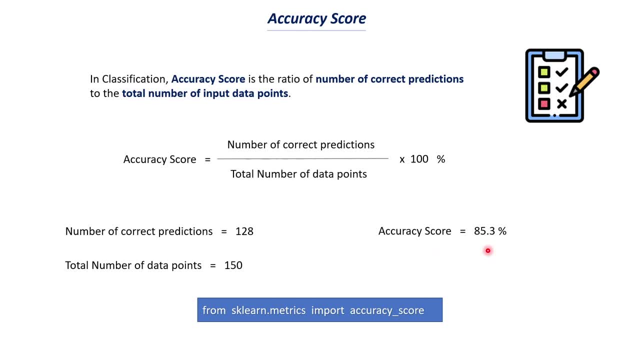 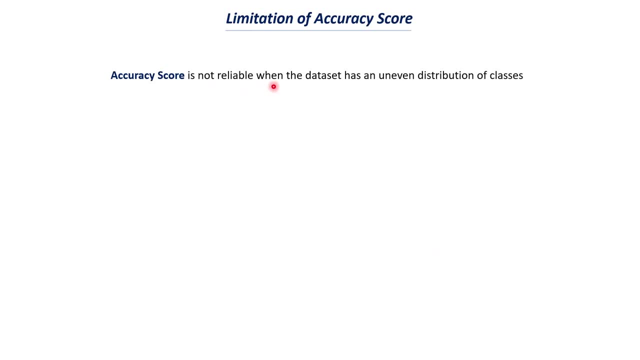 things and we have not, like we have seen that this is how we can quantify the performance of the model, but there is, like, one significant limitation to this: accuracy score. so accuracy score is not reliable when the data set has an uneven distribution of classes. so this is very 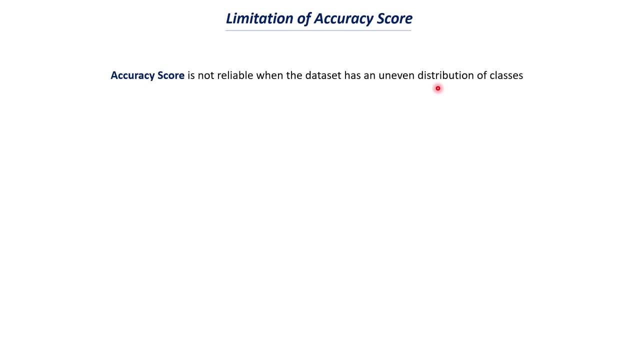 very important. let's say that we are training our model to predict whether a person has r disease or not. so this is again two classes: person with our disease, person without our disease. let's say that the total size of the data set is like a thousand if there is like an uneven distribution. 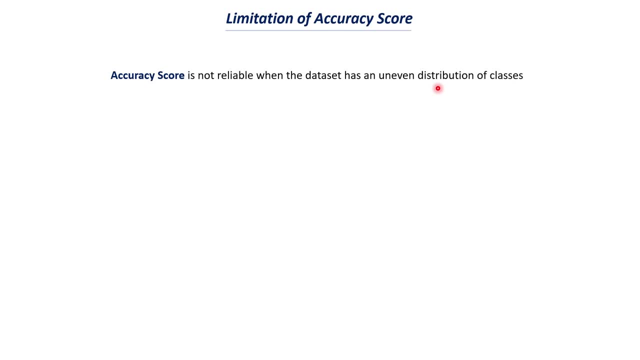 in that case, accuracy score can be misleading. okay, so we cannot rely on accuracy score? let's try to understand this with an example. so let's say that we are building some deep neural network in order to predict whether an image represents either a dog or a cat. okay, and the total number? 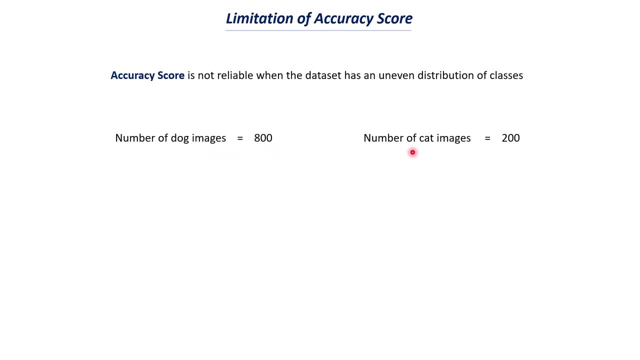 of images we have in the original data set are 800 dog images and 200 cat images. okay, as we can see, here there are two classes. first class is dog and the second class is cat. here, as i told you, there are two classes, so there is a number of images and the number of dog images is very high compared to 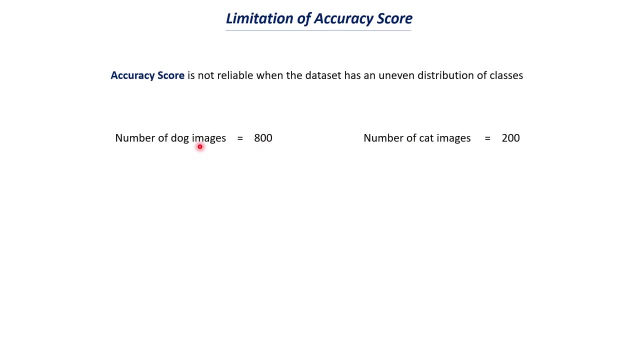 the cat images. so this is the distribution of classes. so it is like four is to one, ratio of dog images to cat images and, like the dog images is you know, the number of dog images is very high compared to the cat images. when we have a data set like this, if we train our neural network or 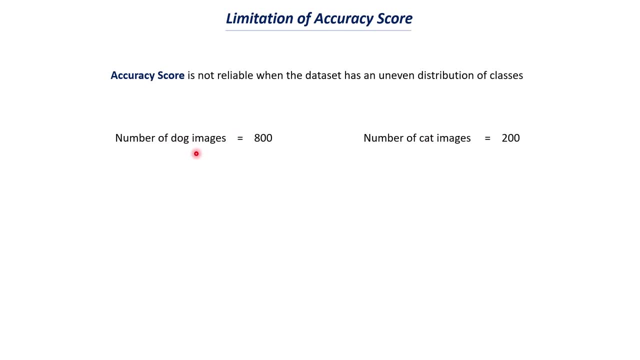 any machine learning model with this kind of data. the machine learning model cannot understand the difference between a dog image and a cat image, just because the number of images for one class is very cat images as cat. so this is the problem with uneven distribution of data. so let's say that 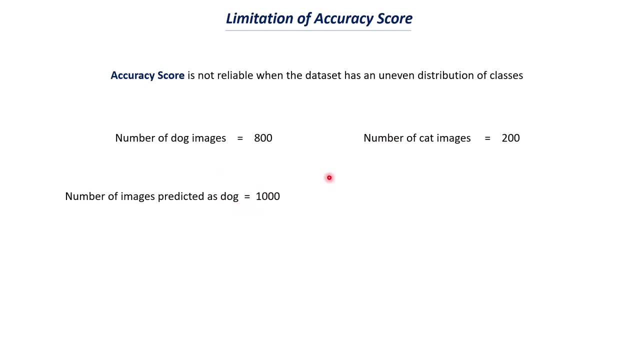 the number of images predicted as dog is thousand. so we have, let's say that we have, trained our neural network with this thousand images and we are, like, again predicting. you know, using this neural network, we are predicting with the training data. let's say, this is our training data, which is: 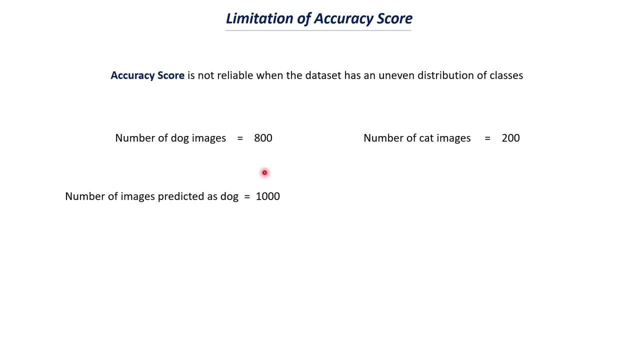 800 dog images and 200 cat images, as i have told you. as there are, you know, there is like insufficient amount of cat images. all the images will be predicted as a dog, so there is a possibility for this. so let's say that out of thousand, all the images has been predicted as dog, if you calculate. 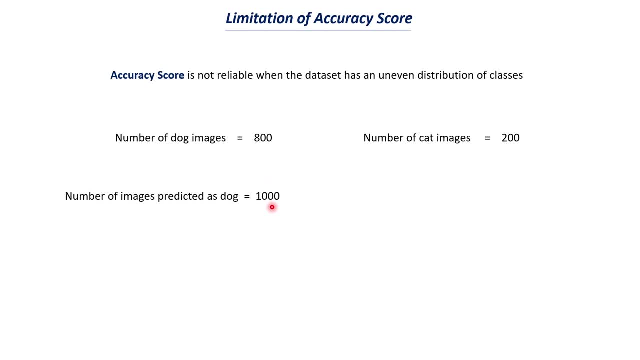 the accuracy score in this case. let's see what is the value that we are getting. so the number of images predicted as cat is zero. obviously, because all the images are predicted as dog. so the number of correct predictions in this case is 800, right, because, obviously. so, out of the these thousand, 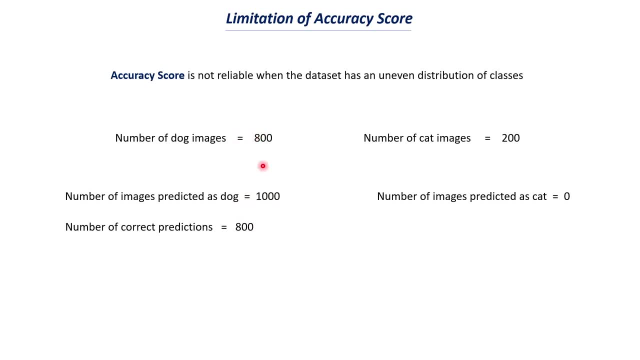 images 800, or dog images, so we will consider these as correct predictions, whereas the total number of data points in this case is thousand. so if you want to find the accuracy score, we will divide it by 800, divided by 1000, into 100 percentage. so this: 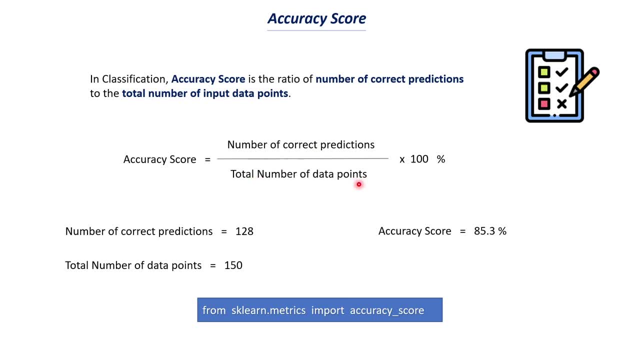 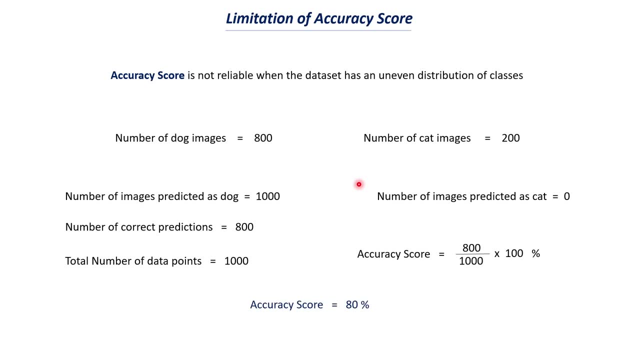 is what we have seen before: number of correct predictions divided by total number of data points. and this is what we get: 800 divided by 1000 into 100. so the final accuracy score that you get is 80 percentage. okay, right, so we can say that 80 percentage is a good accuracy score, right? 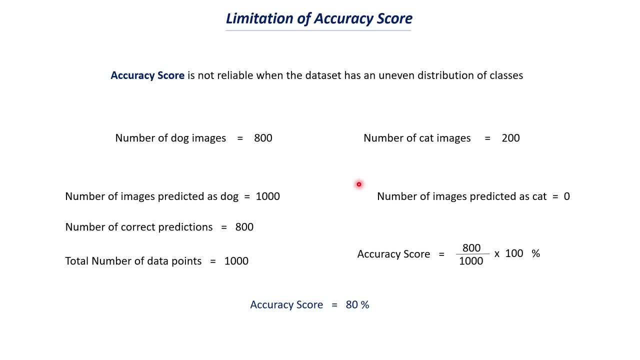 but this is not a good performing model. so this is actually a, you know, an underperforming model. let's try to understand why. so we are going to use this trained model that has been trained on uneven distribution of dog images and cat images, and now let's say that we have a different test. 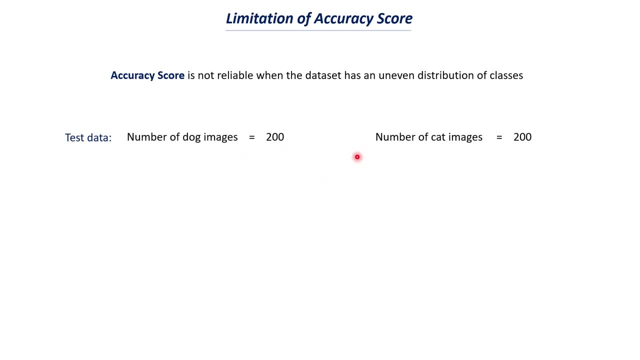 data and in this test data there are 200 dog images and 200 cat images, right, and the model hasn't seen these images before. so when you use that model, which is trained on uneven distributed dataset, if you use that particular model, again all the images will be classified as dog because the 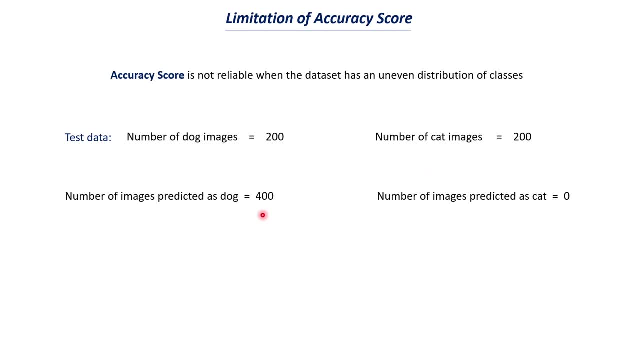 understand how a cat image looks like. so out of these like 400 images, so there are like 200 dog images and 200 cat images. all the images will be predicted as dog by our machine learning model and no images will be predicted as cat. so in this case, the total number of 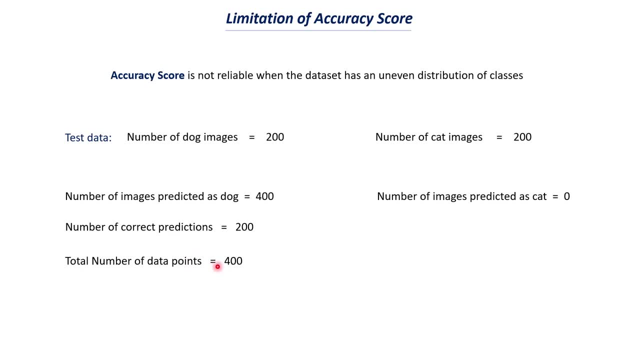 correct predictions is 200 and the total number of data points is 400. right, because out of these 400, 200 are dog. so 200 are obviously correct and the remaining 200 are wrong. right, so the total number of correct predictions is 200 and total number of data points is. 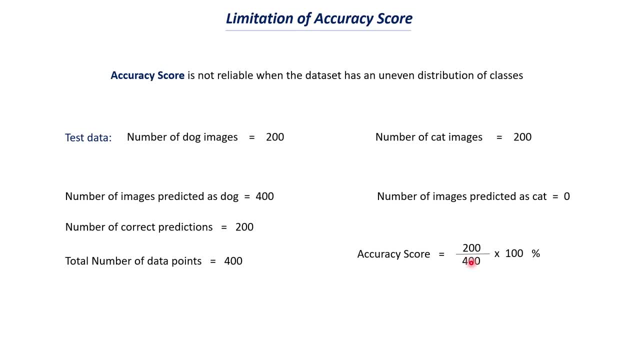 400 in this case, if we try to find the accuracy score, it is correct predictions by total number of data points, which is 200 by 400. in this case, the accuracy score is 50 percentage. so there is like a huge difference between this accuracy score, which is 80 percentage, and 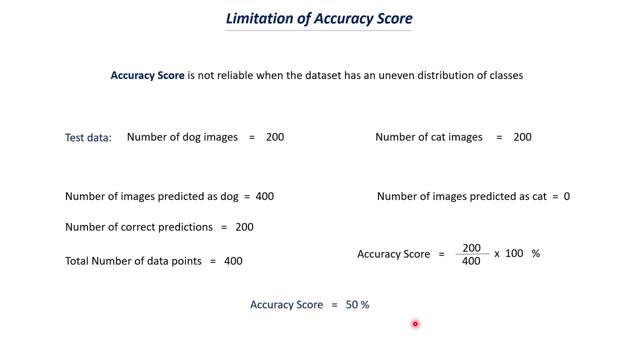 this accuracy score. so this is why accuracy score is not reliable when there is an uneven distribution of data. okay, so if there is like like let's say that in the training data there are like an uneven distribution, in that case we make it an i accuracy score. but it is actually a wrong score because all the images are predicted as. 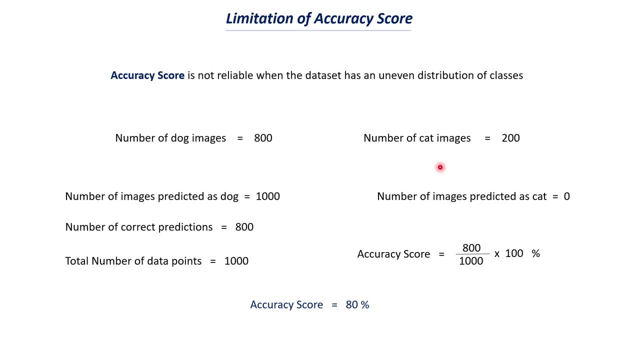 cat, so we can say that the model is not performing well and we can capture this. you know, incorrect performance of the model when only like when, we have a data set like this, where the distribution is kind of even so, this is where the matrix like confusion, matrix, like confusion matrix, or 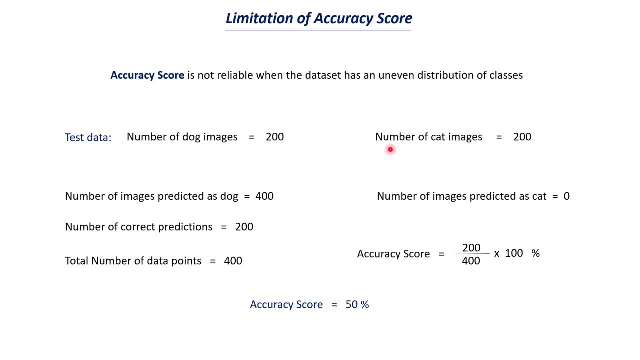 precision and recall comes into play. so in this video let's try to understand how confusion matrix kind of builds us in order to understand this- uh, you know this- this limitation of this accuracy score, and how we can use that efficiently. in the next video i'll explain you about this. 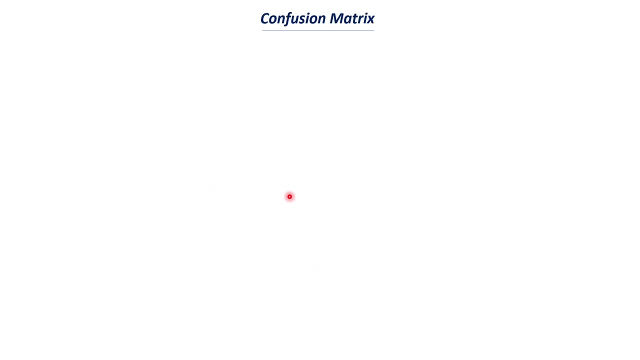 precision and recall and all those things. so let's discuss about this confusion matrix now. so confusion matrix is a matrix used for evaluating the performance of a classification model. so again, we can use this only for classification model and it gives more information, information than the accuracy score. so, like, let's say, what is that particular? 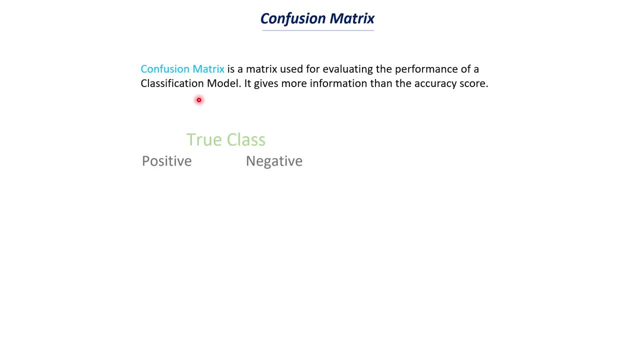 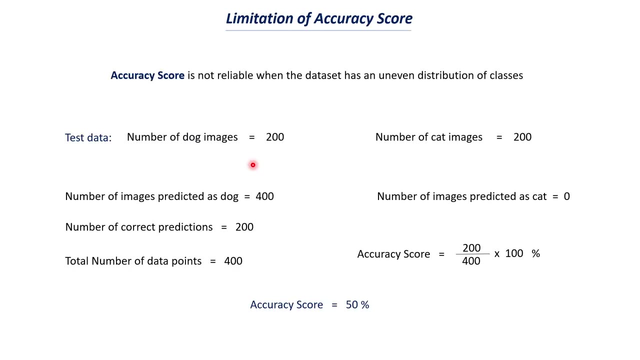 information that is, uh, you know, helpful for us. let's say that this is the true class of the data points, so positive and negative, and this is the predicted uh class. so in this case- the previous case- the two classes are dog and cat. so in this case, we are considering as positive and negative as the two classes that we have. so this: 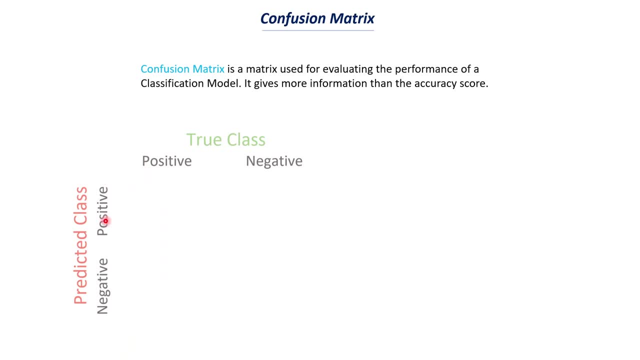 is the two true class, so true labels, and this is the value predicted by our model. let's say that we are uh not doing this for coven 19 test cases. so let's say that, uh, there is some, some tests like, uh, rtpc or or. 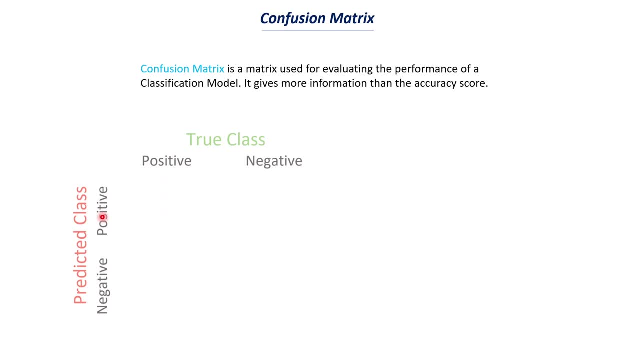 this: uh, rapid antigen test. so we have this: two tests for, uh, covid 19. let's say that, uh, we have this true class and predicted class. so true classes, whether a person is, uh, you know, really having this covid 19 infection, and predicted classes. let's say, uh, you know the values predicted by our model. so 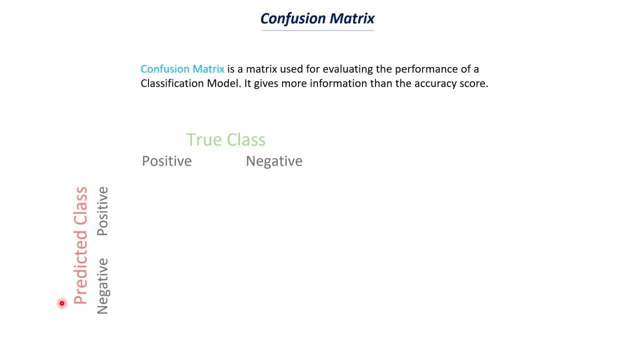 let's say that we are building a ml model that can predict whether a person has covid 19 infection or not, based on certain symptoms. so let's consider this. so the first- uh, you know- quadrant of this confusion matrix represents my true positive. so what does what does this true positive means? is so the true class of the person is positive? 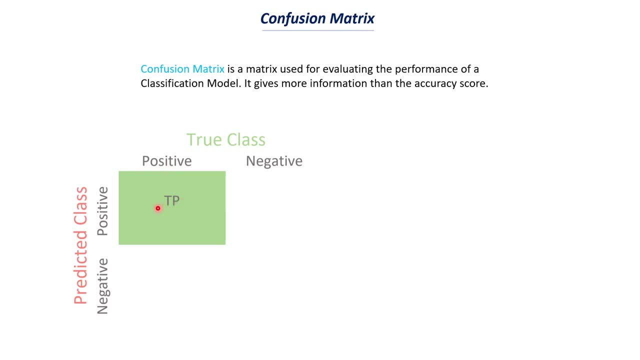 that means a person actually has a kobe 19 infection and the model also predicted correctly. so you have to see this uh label and this label. so this is my true class and this is my predicted class. so both these things matches right, so we can say that this is my correct prediction. 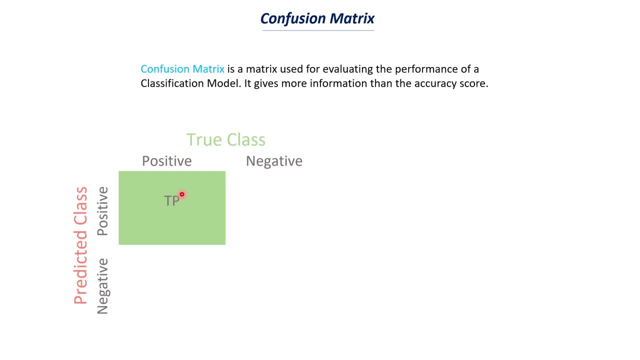 so what this basically means is: a person really has proven 19 infection and the model has also predicted correctly. and what does the second box represent? is true classes negative. that means a person doesn't have any kobe 19 infection, but the model has predicted that the person has kobe 19 infection. so this is what we 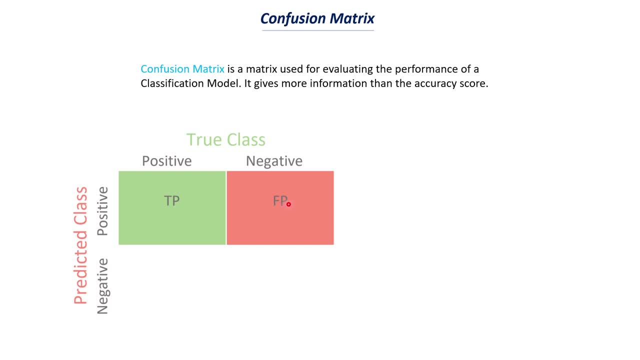 call as false positive because, uh, this positive is not correct one, so this is an incorrect one, whereas we call this as true positive, which is represented as tp, because the person is actually positive and the third contract in this case is false negative. so in this case the true class is positive, which means a person has kobe 19 infection, but they have been predicted as 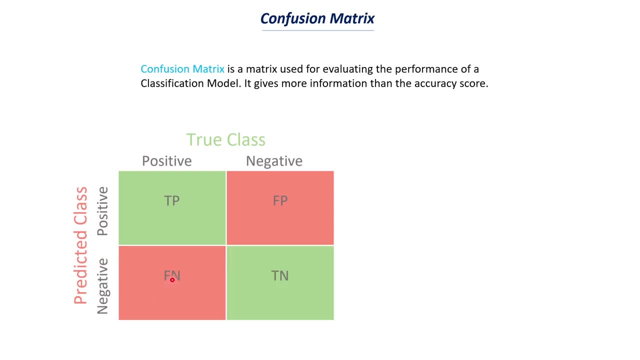 So this is what we call as false negative and the final quadrant is true. negative. So the person does not have COVID-19 infection, so they are like really negative, but the model is also so the model also predicted as negative. so this is what we call as true. 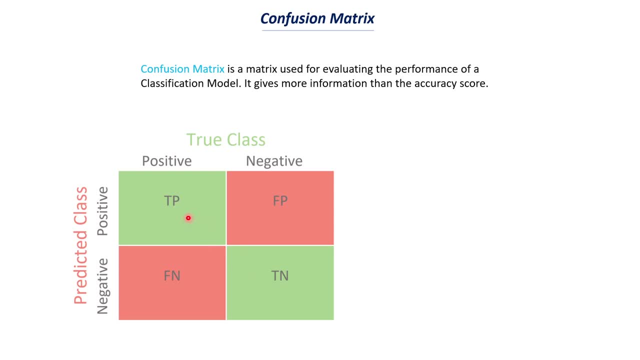 negative. So these two green color boxes represent my correct predictions and these two red color boxes represent my wrong predictions. So true prediction is nothing but so. TP means when a person is tested positive for COVID-19 and the model also predicted correctly that they have infection. 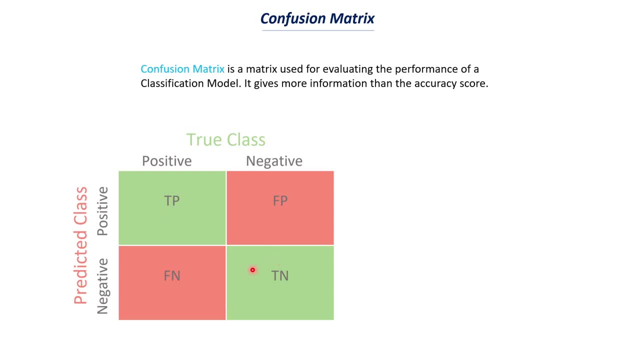 So it is called as true positive, and what is meant by this true negative is that a person does not have COVID-19 infection and the model has also predicted correctly that they are negative for COVID-19 infection. So these two are my correct predictions, and false positive is something when a person 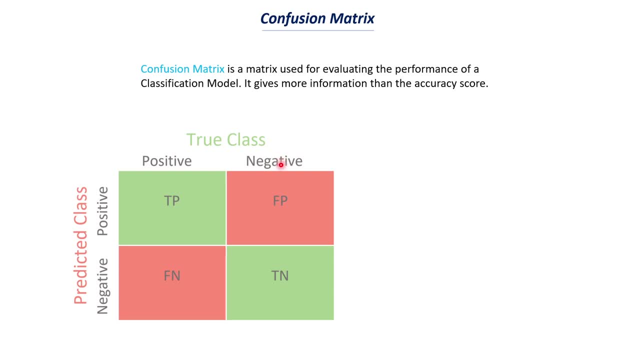 does not have any infection. So we have this: true class is negative, but the model has predicted it as positive. So we have this as false positive. and finally we have this false negative, which means like a person actually has the infection, But the model is predicted as negative. 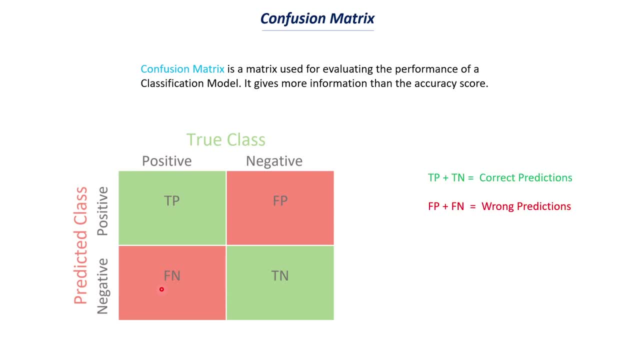 So the model has predicted that the person does not have any infection. So TP plus T and count represents my correct predictions. true positive and true negative represent my correct prediction and false positive and false negative represent my wrong predictions. and you can use this sklearnmetricsconfusionmetrics in order to, you know, use this confusion. 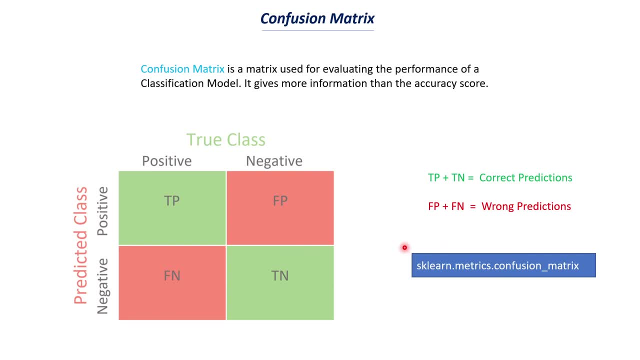 matrix. We will also discuss how we can implement this in python and again. so this is a very important concept that you have to understand. So there will definitely be questions on this particular topic in most of the machine learning and data science interview that you attend. 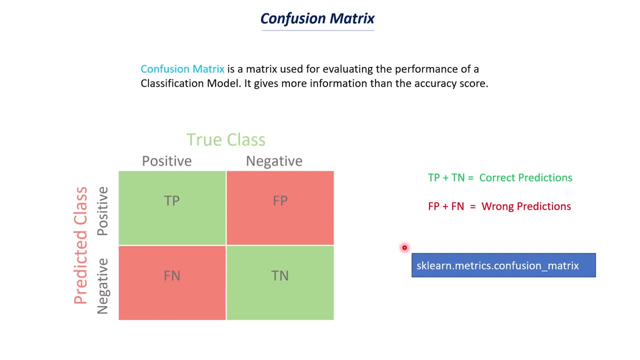 Okay, So the easiest way to understand is by you know, through this covid-19 infections or any other, this medical condition because there is like true positive and false positive, false negative and true negative cases Like these terms are used in the clinical field as well. 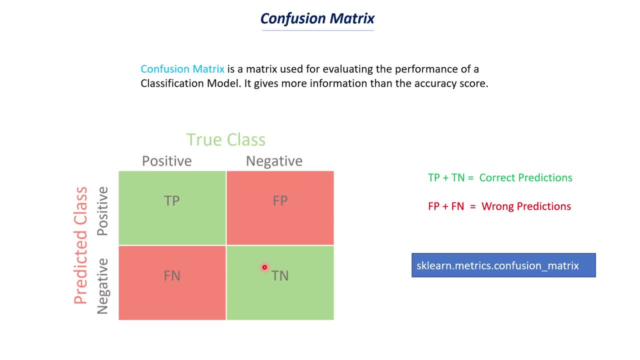 So this is how, like, they kind of represent people who have been tested positive, If they are, you know, if they do not have any infection, and things like that. So this is an actual term that is used in the clinical field. this is what we use in confusion matrix as well. So the advantage of this confusion matrix is: 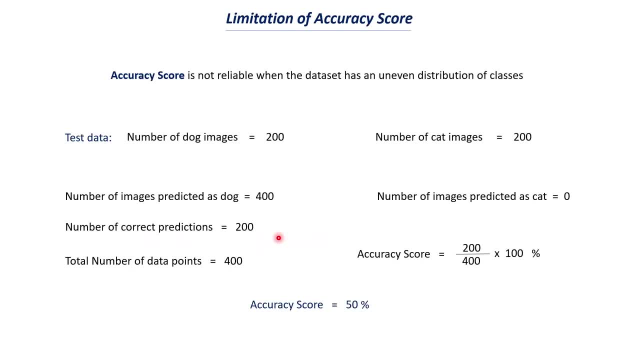 even like when there is this undistributed, like uneven distribution of classes, even though there is, like this, i accuracy score. So in this case we know that the accuracy score is i, but when you implement a confusion matrix, in such cases we can clearly see whether the model is. 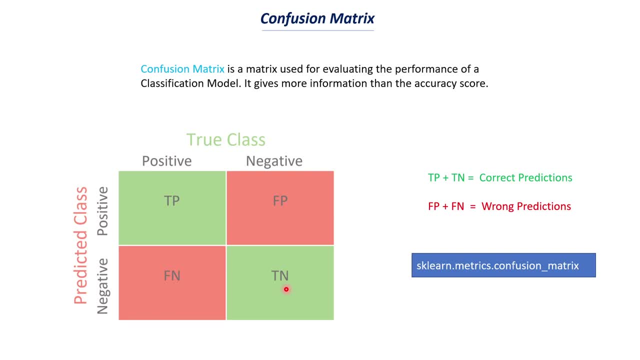 making good predictions or whether all the models has been predicted. as you know, one class. So this is how confusion matrix will be helpful for us. and now let us try to understand how we can kind of implement this in python. So I will open my google collab. So I have this code already. 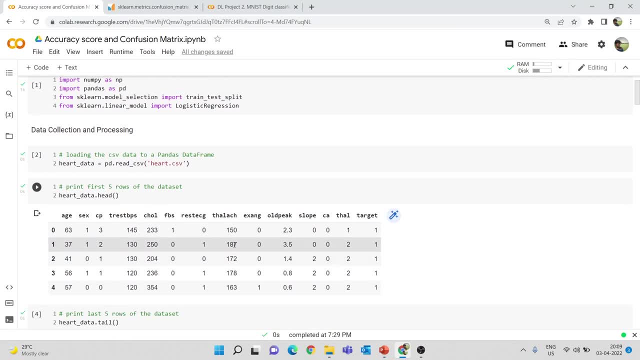 already. So the data set in this case that I have used is this art disease prediction that we have used before. I will also give the link for this video, where I have completely explained you how you can use this data set in order to predict whether a person has this art disease or not. 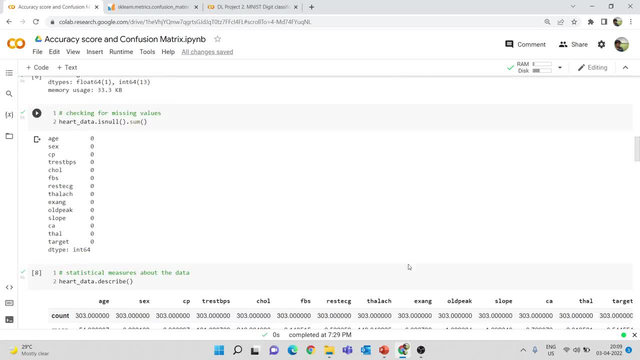 So I am not going to go into all these details. Let us directly come to this model about the data set. So let us go to the data set. So let us go to the data set. So let us go to. 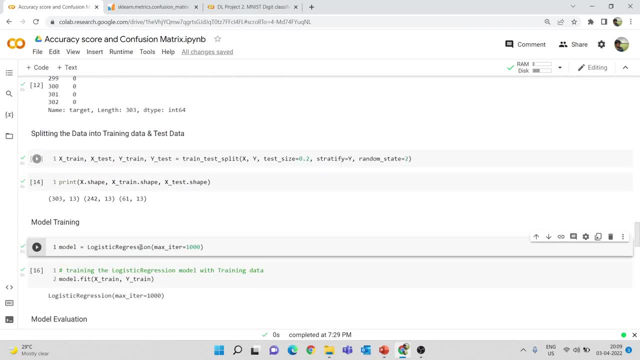 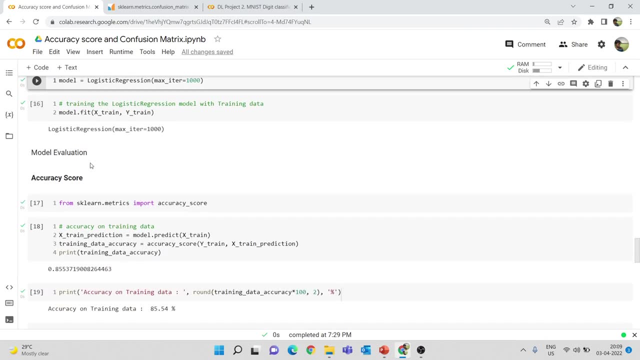 the evaluation part. So we have processed this data set, splitted it into training data and test data and we have trained our logistic regression model with this x-train and y-train. So this is my model evaluation part and I am going to calculate my accuracy score, So I am importing my 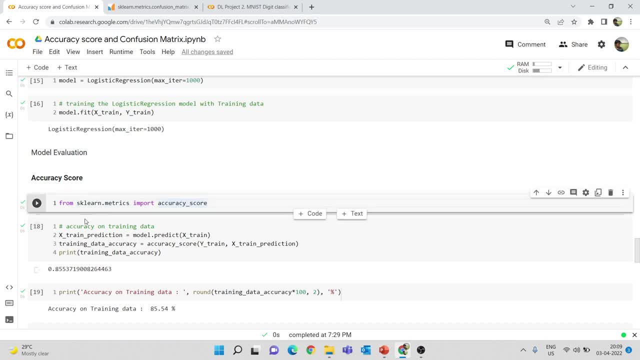 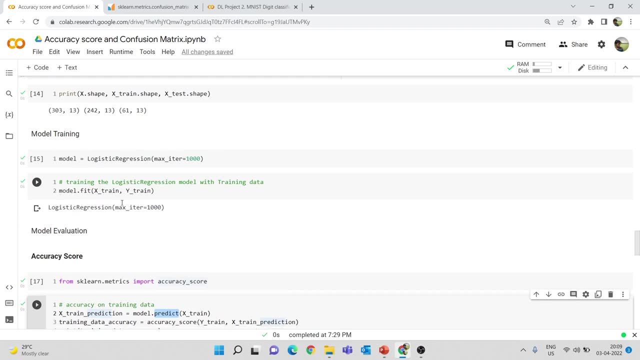 accuracy score function from sklmmatrix and I am creating a variable called as extreme prediction and I am going to predict the values. So model is my logistic regression model, which is trained on the training data and I am predicting the labels for my training data. So extreme prediction is 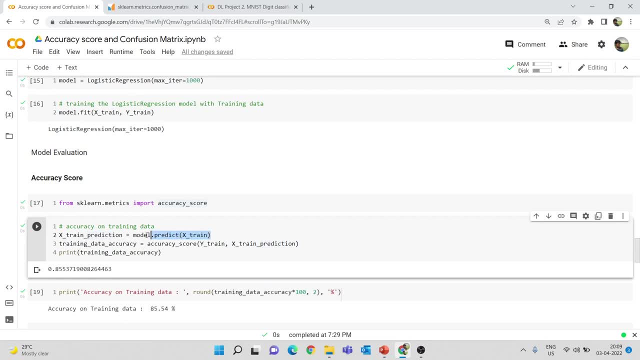 equal to modeltrainmatrix. So I am storing all the predicted labels in this extreme prediction and I am going to calculate the accuracy score So that accuracy score is stored in the variable called as training data accuracy. So I am using this accuracy score function and within this I have to mention the true label and 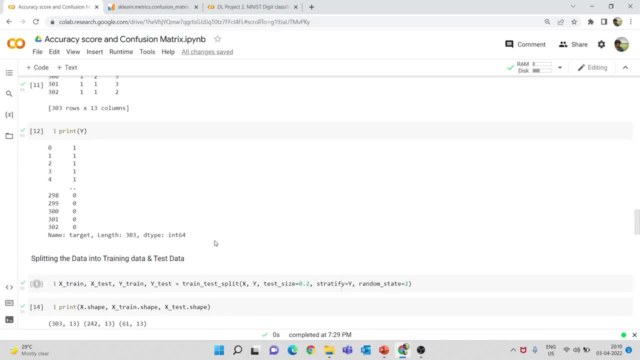 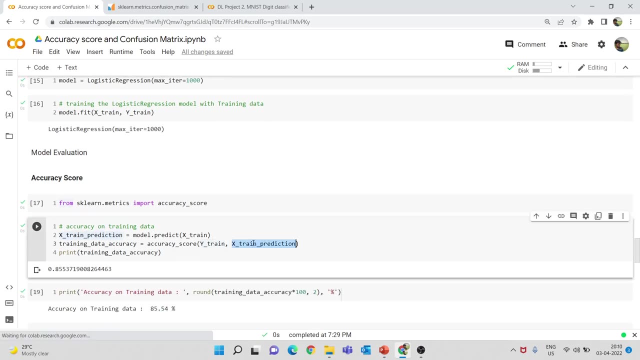 the predicted label. In this case the true label is y-train, which we have obtained from this train test split. So here your y-train, which is my training data prediction, and the prediction made by the model, which is extreme prediction. So accuracy score is equal to x-train. So 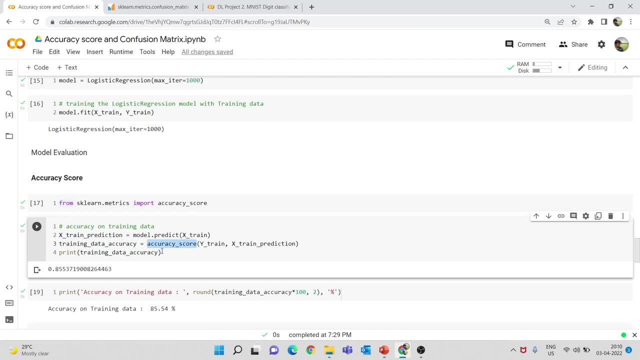 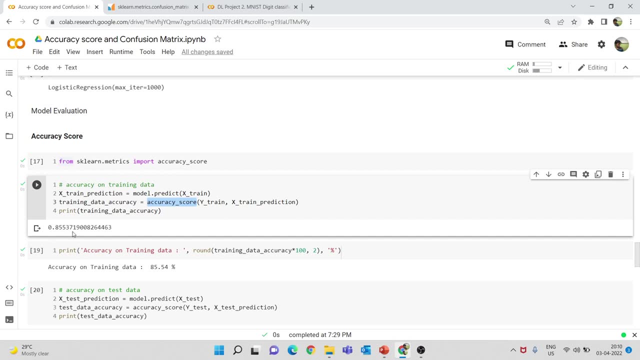 accuracy score will compare these two set of arrays and it will give us the accuracy score. So in this, if I print this accuracy score, the value is 0.8553, which is equal to 85.53%, and if you want to want to round this to percentage, you can use this round. So round will, kind of it is used to. 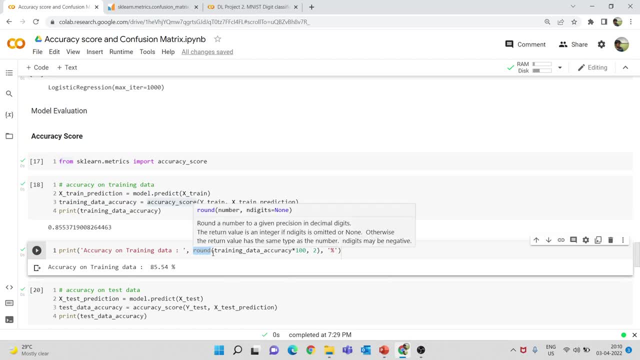 you know, remove some decimal places, or it can also convert, like floating point value, into integers, So it will basically round the values. So what I am doing here is I wanted to round this training data accuracy, which is x-train. So I am going to round this training data accuracy, which is x-train. 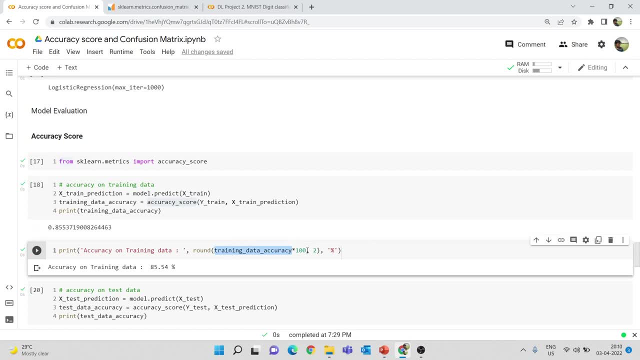 is in this range of like 0.85 or something, so i'm going to multiply it with 100 in order to convert it to percentage. what does this two represent? is: i want two decimal places, i want two decimal values. so if you want like three decimal values, in this case we have to mention three. so this has been. 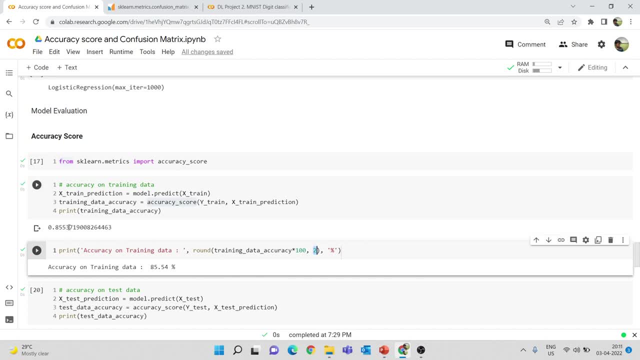 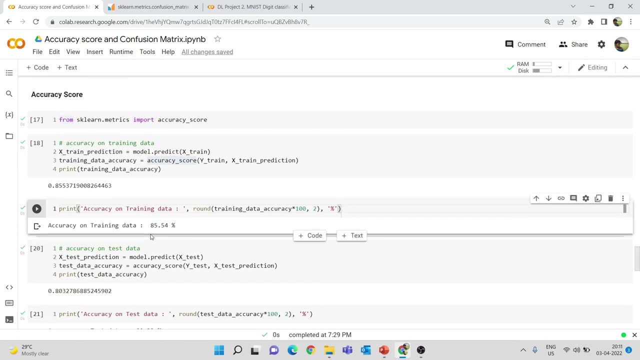 rounded so it is like eight, five, five, three, seven. so this three has been rounded to four, as we have the value of seven in this case and we are adding a percentage symbol to it. so, as you can see, in this case the accuracy score value is 85.54. percentage, which means, um, if you predict uh. 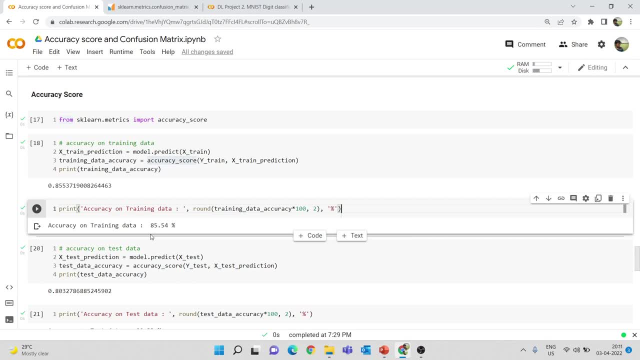 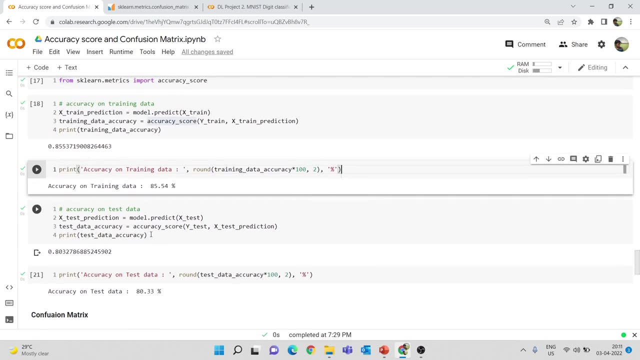 for using this model. if you predict whether a person is having our disease or not for 100 people under data points, the model can make correct prediction for 85 people. so this is what we call as an accuracy score. so this is the accuracy score on the training data and this. 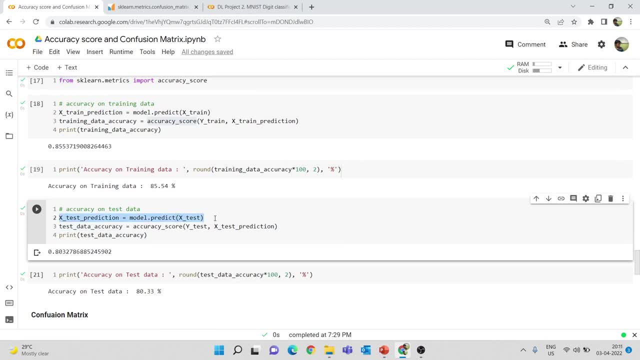 i am just doing the same thing. the only difference is that i am calculating the accuracy score for test data and this accuracy score is, like, very important. the training data accuracy is not that important, but test data accuracy is very important. so i'm calling my x test prediction where i'm storing. 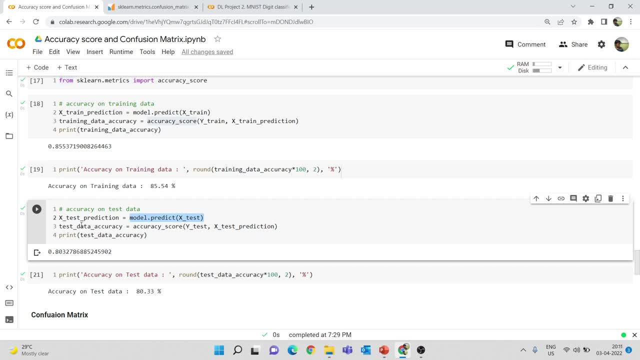 all the predictions made by the model and i'm storing this to x test prediction and i'm using the security score function. so y test comma, x test prediction, so i'm comparing the true test. uh, you know labels and the labels predicted by my model using this accuracy score function and 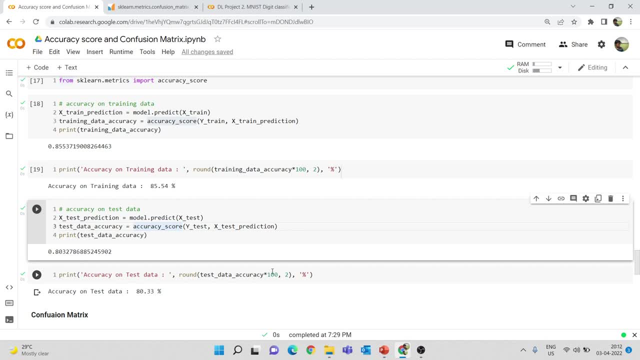 the accuracy score is 80.32 percentage. so when i round this to two decimal places, i'm getting the percentage value as 80.33 percentage. so i'm sure that most of you would know this already. uh, you know calculating this accuracy score. now let's move on to confusion matrix. in order to 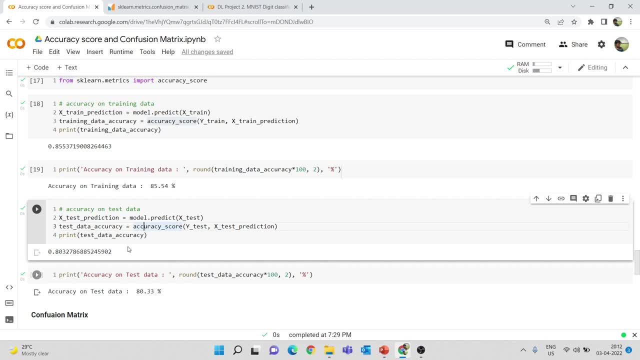 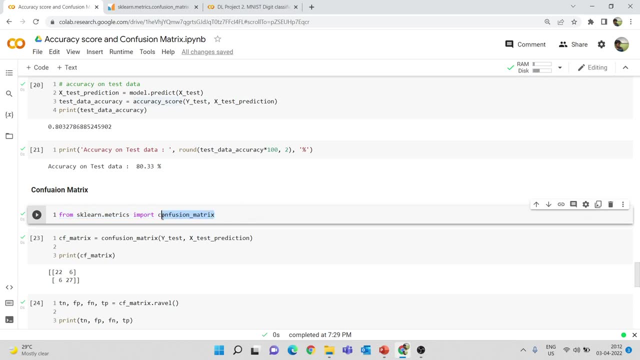 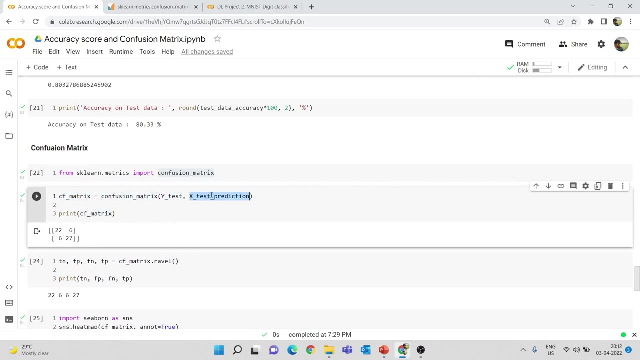 understand that, uh, you know, we can, uh, you know, represent that matrix, uh, using this confusion matrix. so from sklearnmatrix i'm importing confusion matrix, so this is the function in order to calculate this, and i'm creating a variable called the cf matrix. so cf matrix, confusion matrix of y test and x test prediction. so it is just similar to this step. so instead of 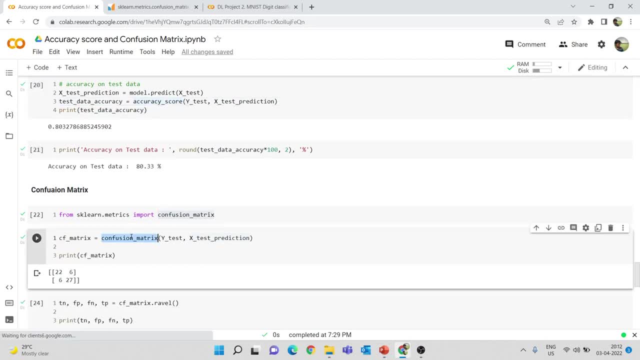 uh, you know, using accuracy score, we are using this confusion matrix function and we are storing this matrix to cf matrix. so, as you can see, the result is stored in a matrix. that's why we are naming this as confusion matrix. i'm creating a variable as a short form of cf matrix, and i'm 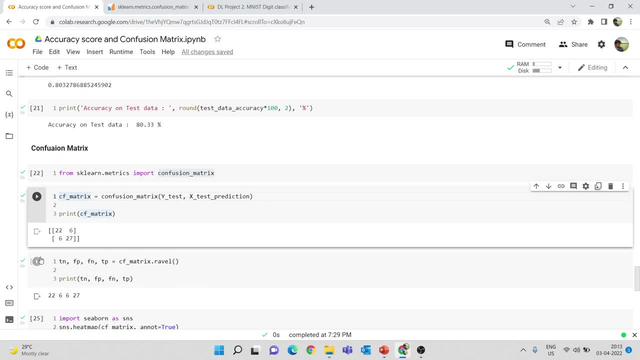 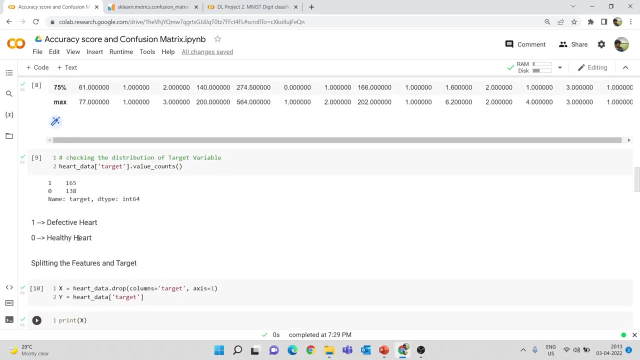 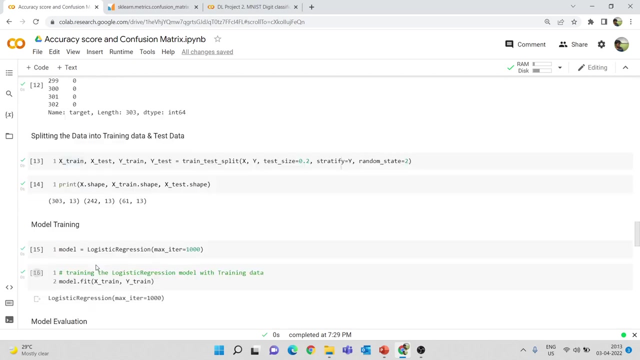 printing it. so this is the value that i'm getting: 22, 6, 6, 27- but we are not sure. what does these values mean, right, uh, like in this case, we have two labels. so the first label is one. one means a person is having r. this is zero means a person doesn't have rss- okay, but in this case we are not sure, uh. 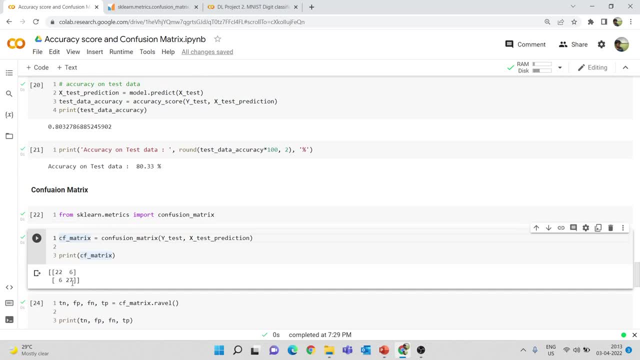 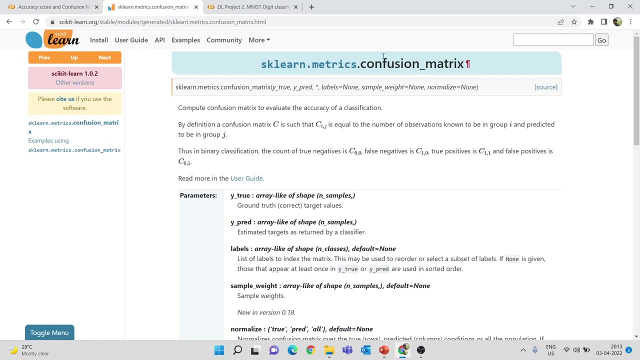 like: does this? uh, 22 means 6 or 27 means. so we are not sure which is true, positive or which is false, negative and so on. you can go to this sk learn dot matrix, dot confusion, matrix, documentation. in sk learn you can see the order here. so in the case of binary cases, binary cases is when you have like. 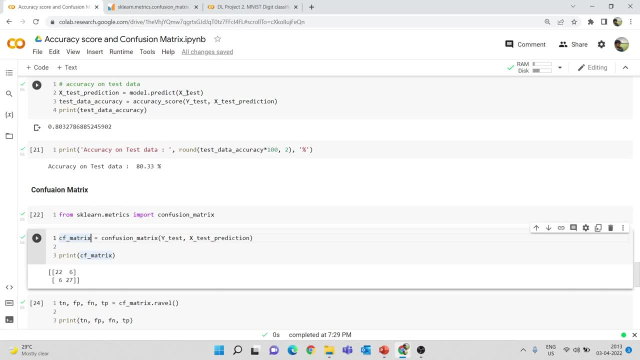 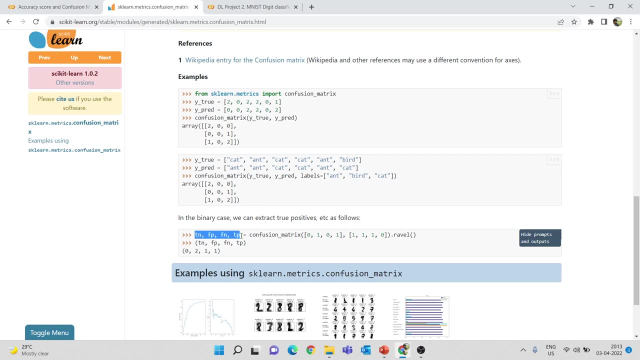 two classes. in this case we have two classes as person with our disease and person without that basis, right? so this is the order: first is true negative and then we have false positive, false negative and true positive. so these are like the order that we have and uh, you can kind. 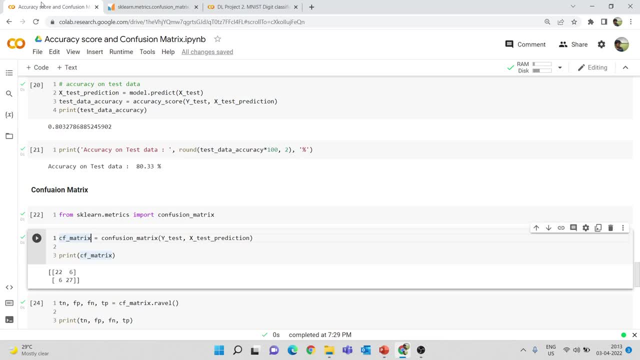 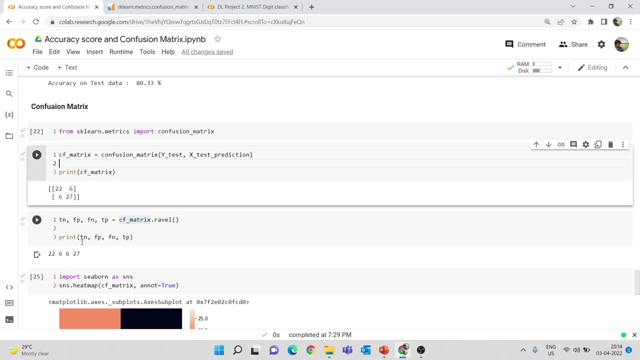 of get this values using this dot travel function, so i'm going to like extract these values using the cf matrix, dot travel, cm matrix is where i have scored my confusion matrix and we will get all this true negative value, false positive value, false negative value, true positive value. so this: 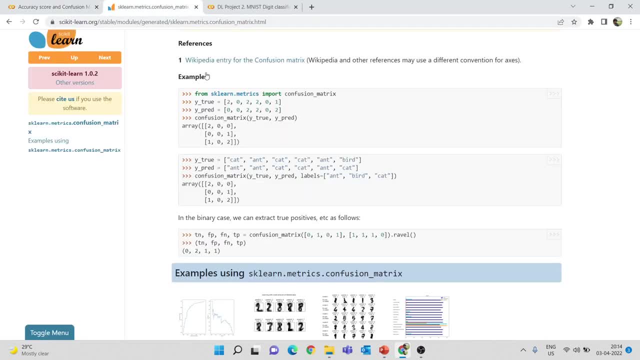 is how you can extract all these values. and also, the other important thing is, you can also, you know, build this confusion matrix for a multi-class classification problem. if you have a multi-class classification model and it's called multi-class classification, you see, in this one they have like multiple classes and bird and cat, whereas in this case 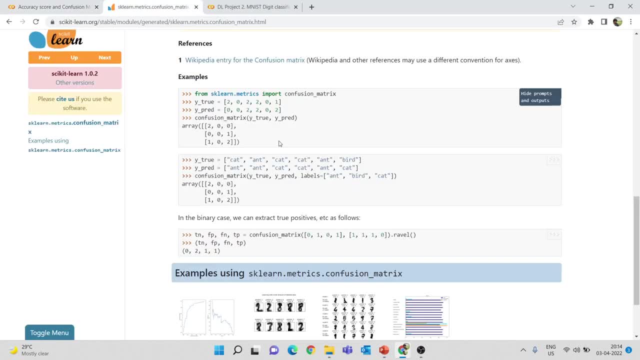 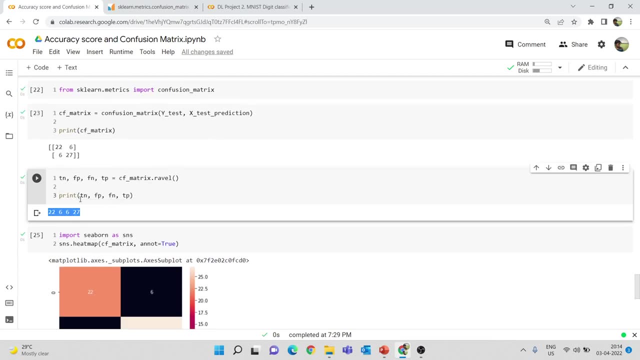 we have only two classes, so you can also use this confusion matrix for multi-class classification problems as well. and if you are not sure, on what does this number represents? and if you want to represent this in an eat map, that is also possible and it is like a more efficient. 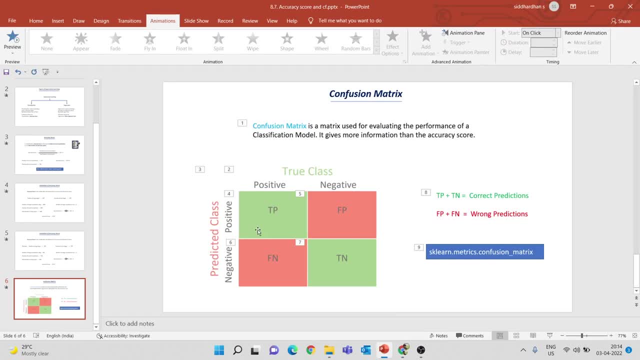 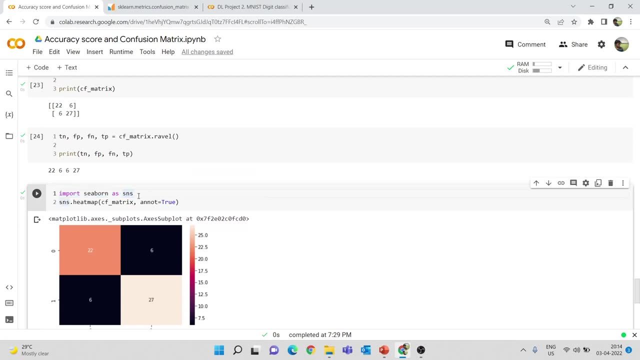 way in order to understand this confusion matrix. so it is like similar to how we have built this confusion matrix here, so you can import this c-bond library, as we know that this is a data visualization library, and we are going to load this confusion matrix in the form of a eat map. okay, so i'm calling this snseatmap function and the parameter. 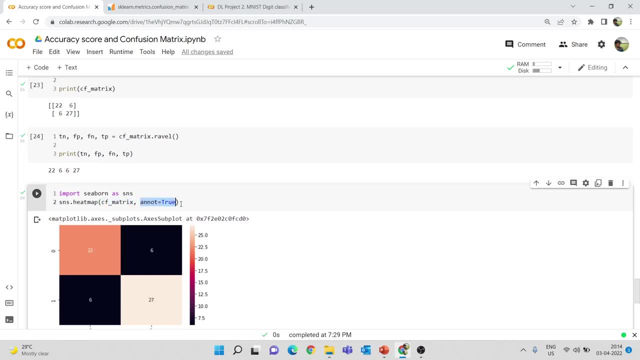 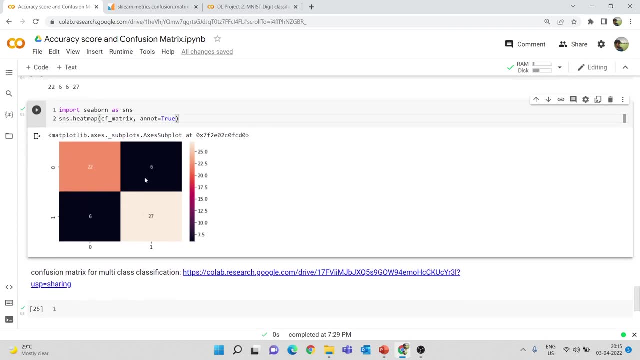 i'm passing is my confusion matrix and the annotation is equal to true. so, like i want these values, so label value. so that's what this annotation means. now let's see what does this confusion matrix this particular eat map represents? so we have the value zero here. 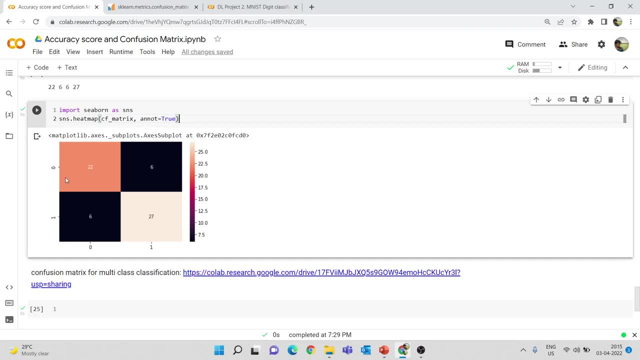 also, we have the value zero. so this means my true prediction. so you can just see this: uh, you know, label in the y-axis and the label in the x-axis. if both the things match, that is my correct predictions. so in this case, zero. let's say that this is this is my true. 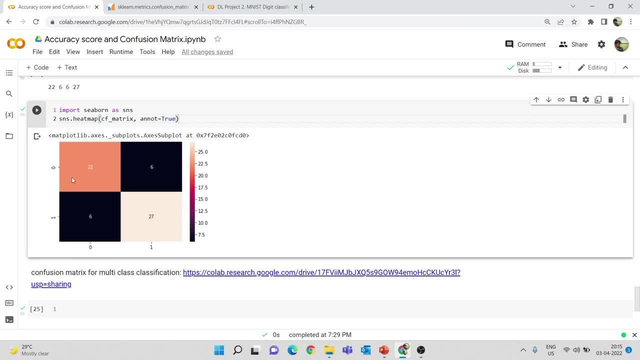 class: okay, true label, and this is my predicted label. so, in this case, what does this 22 means? is like, uh, 22 data points as the label 0 and all those 22 data points has been classified as 0. and this 27 means is like those 27 data points as the label 1, and they have been predicted. 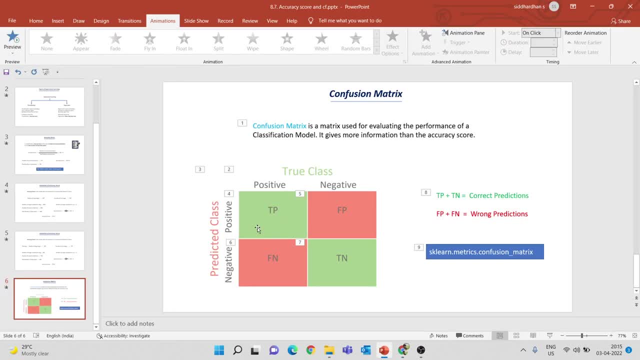 as the label 1. so these are my correct predictions. so these are the green colored boxes represented here. so you just have to see the label in both the sides. here it is positive, where it is also positive. so we have like green color here, which is the correct prediction. so in this case we have positive and negative. so 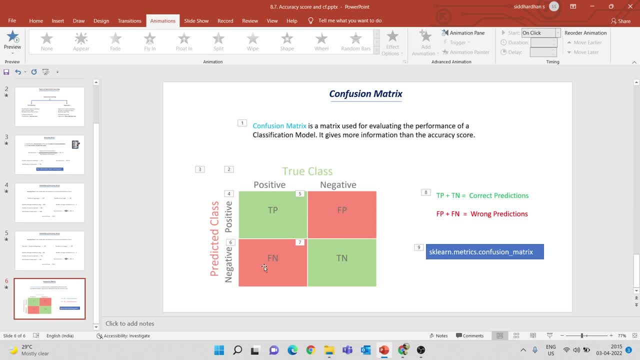 that is like a mismatch in the classes that we have in this case. so this is a wrong prediction. in this case, if you see, in this third quadrant we have negative and positive, so it is a wrong prediction. so here, if you see, this is negative and this is also negative, so this is a true. prediction. so that is the idea here. so here we have the value of zero and positive. so this is a true prediction. so that is the idea here. so here we have the value of zero and positive. so this is a true prediction. so here, if you see, this is negative and this is also. 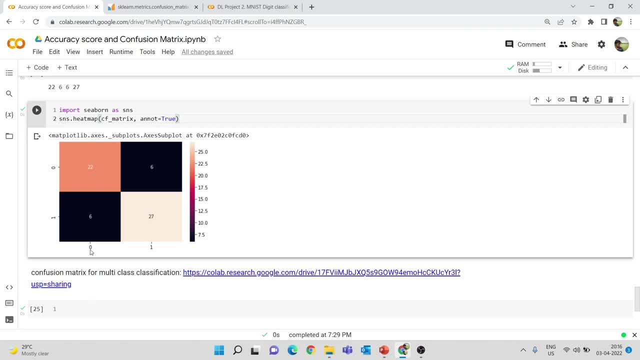 negative. so this is a true prediction. so that is the idea here. so here we have the value of zero. or in the x axis for this quadrant, the, here also the value is zero. so this represents this, 22 represents my correct prediction and in this case one represents like: uh, here we have one, here also. 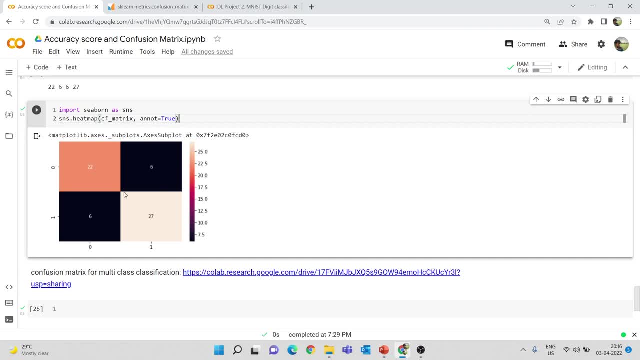 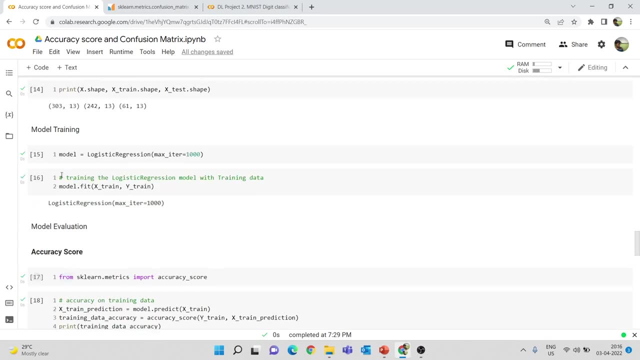 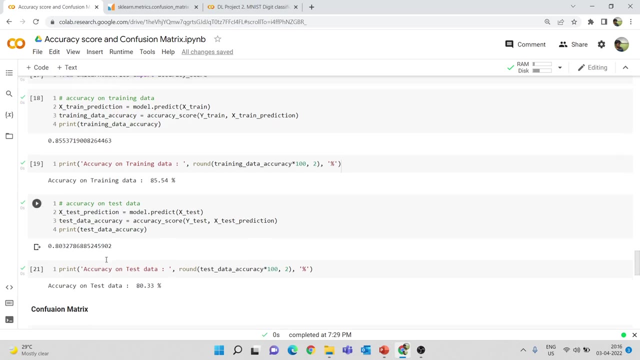 we have one. so 27 is my correct prediction and the six and six are made wrong prediction. so what this means is like, uh, six people who, uh, you know. so let me go to the zero. let's try to understand what the zero means. so zero is lp. at lp admins, a person doesn't have r. this is right. so this is six means. 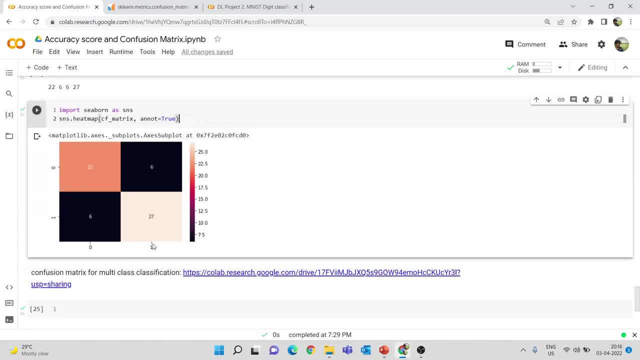 six people doesn't have r. this is, but they have been predicted as one. so if you see this quadrant, you have to just see the uh horizontal label and the vertical label. so if you go here, this is my zero and this is my one, so there is a mismatch. so people doesn't have r. this is has been predicted. 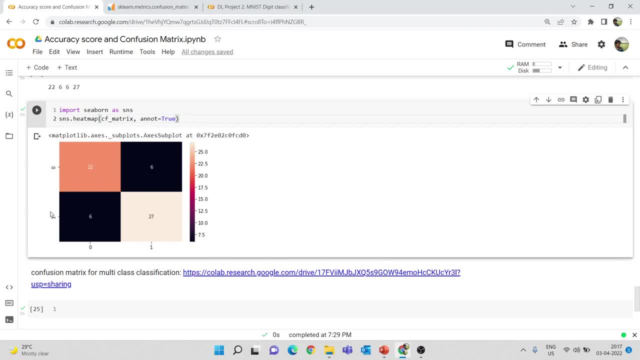 as people with r. this is so. there are like six, uh, wrong predictions in this case and in this case, like people do have r, this is so- we have the label one and they have been predicted that they don't have r. this is so. these two represent my wrong prediction, so you just have to see the labels in. 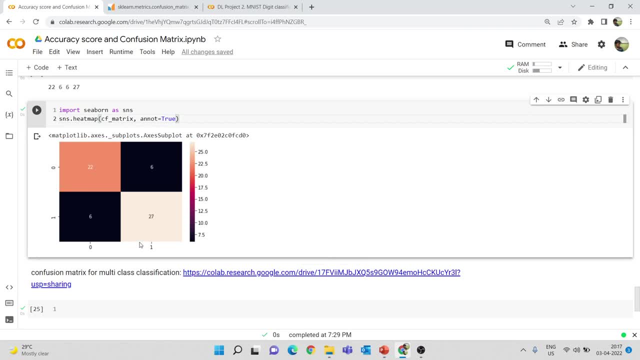 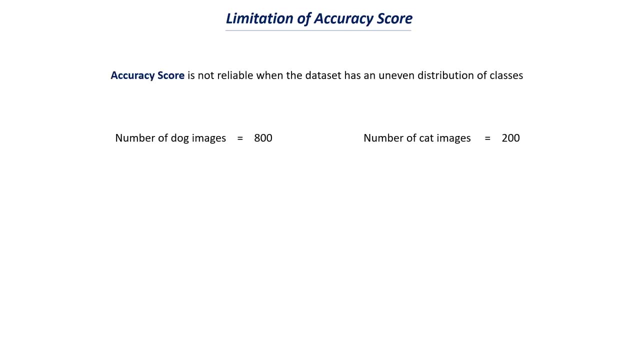 the uh, x, y axis as well as the x-axis, and you will know which are the correct predictions. so, when there is like a problem like this, so we have seen right. so when we have a problem like this, when there is a chance that the data is undistributed, even though the accuracy score, 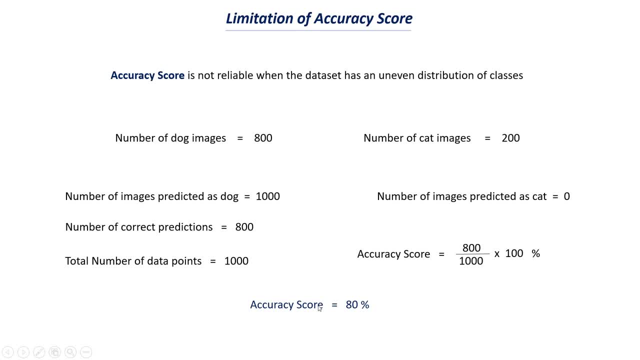 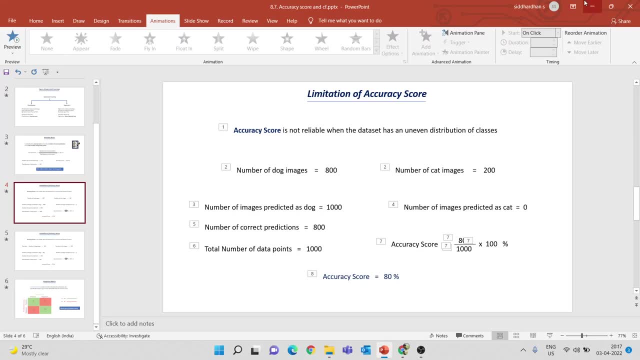 is kind of high. you can try to build this confusion matrix and eat map to understand whether the model is, you know, making good prediction, or all the values has been predicted into only one labels. okay, so that is the importance of this confusion matrix. so in that case, uh, the model will be predicted. 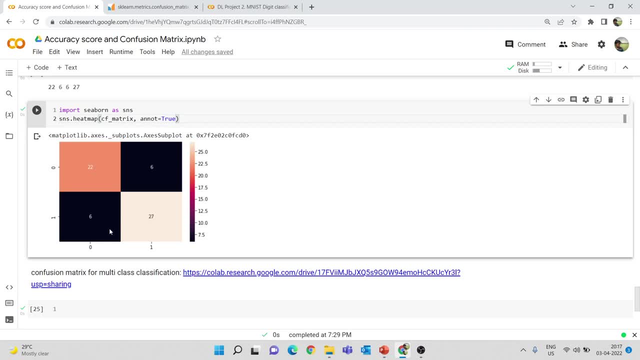 in predicting like: uh, only zero will be predicted in both the cases. no prediction will be made for the class one. so that is what happens for this uh. you know uneven distributed data and that is where we use this confusion matrix and again we have also metrics like precisions and report. 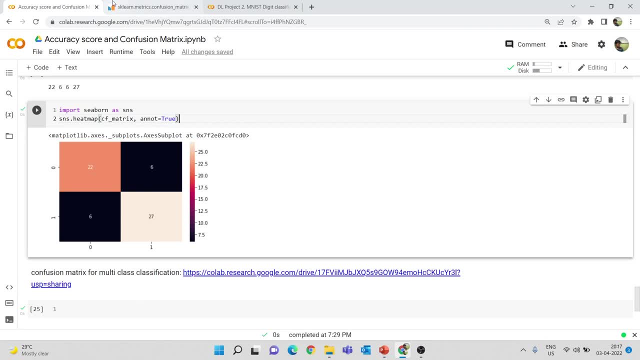 which we will discuss in the upcoming video. so this is for only binary classification problem, right? you can also again use this for multi-class classification, also when we have like more than two labels. and i have another example for you and i'll share this: uh, google collab file link in the 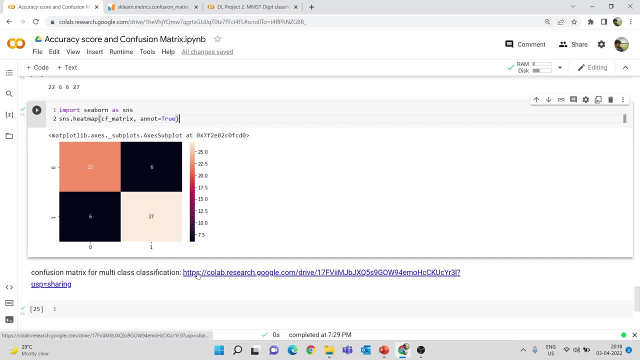 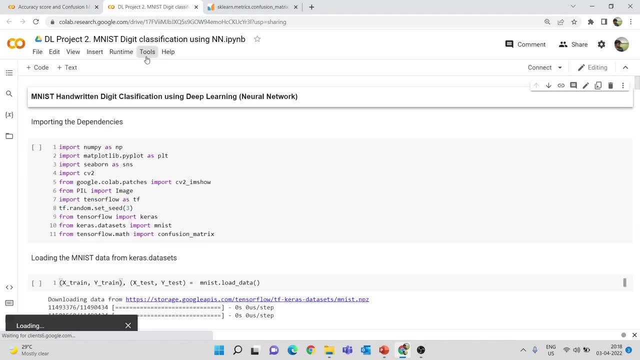 description of this video. you can check that out. i have given a link of a collab file which is again an example for multi-class classification problem. so we have already worked on this in our channel. so this is the mr ist and written digit classification using neural network. i'll also 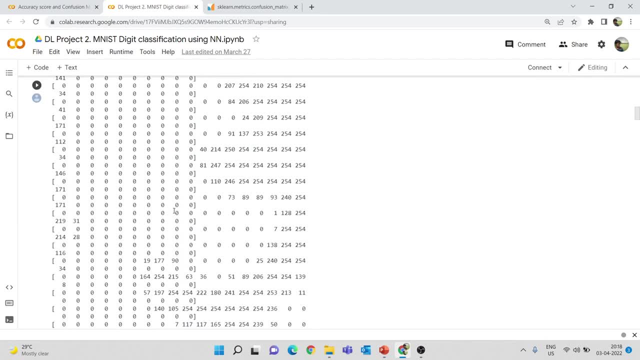 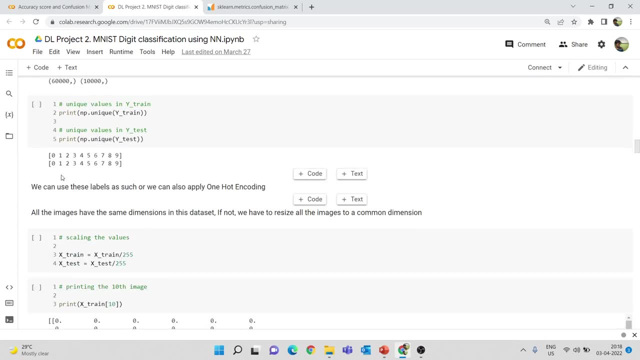 give the link for this video in the description as well. so we have worked on this. so here we are, predicting whether an image, uh, like what is, uh, the digit represented in the image. so the images that we are considering now ranges from 0 to 9, whether it is 0 or 1 or 2, all the way up to 9. so this is. 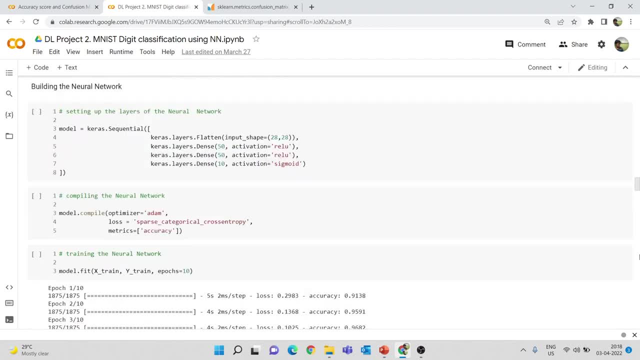 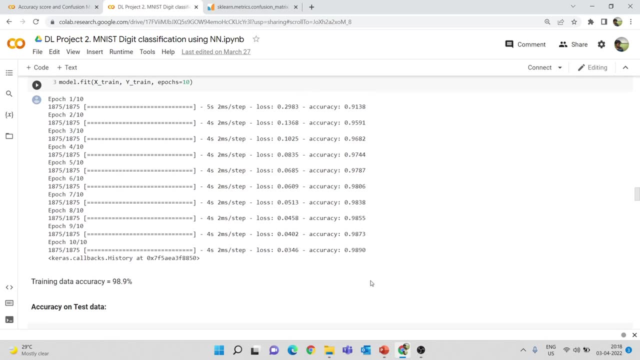 what we are predicting and here also we can build this confusion matrix. so here. so this is the accuracy on the training data, which is 90 like 0.989, which means like 98.9 percentage. so this is my training data accuracy and you can get this test data accuracy using this evaluate function. 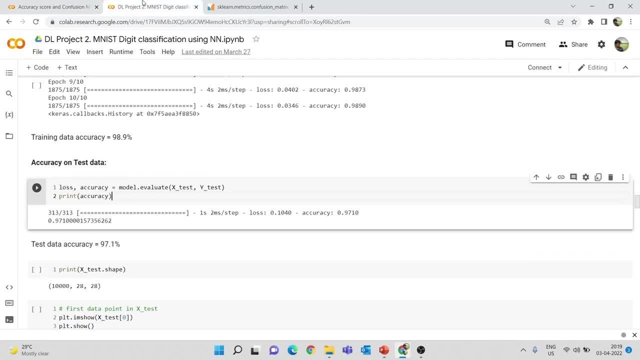 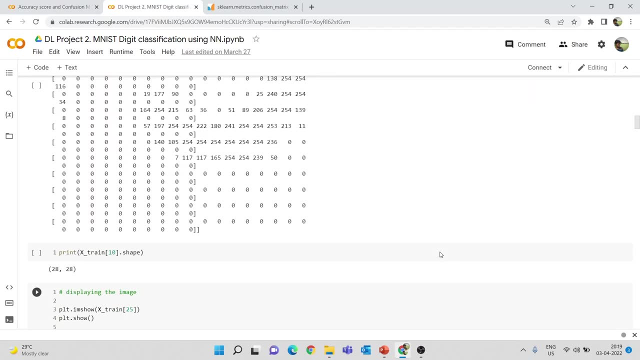 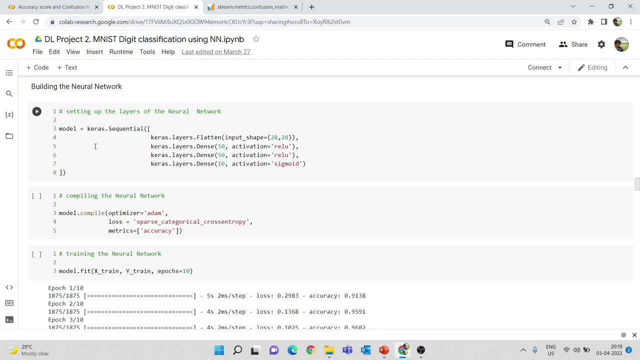 when it is deep learning problem. okay, so this is when we use a scale and models. this is when we use, like neural network from keras and tensorflow. so here we are building this neural network using this, you know, sequential from keras. so let me just open this. so, yeah, so we are building a neural network using keras, and when you do that, there is a function. 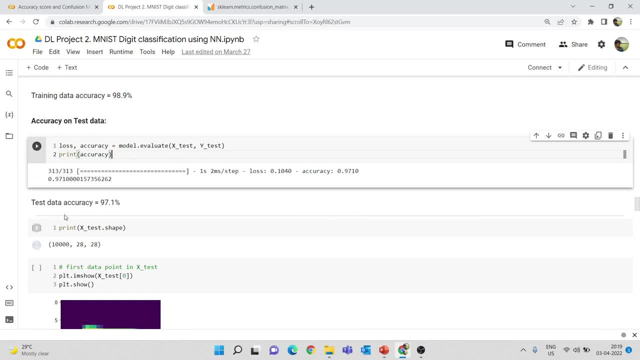 called this evaluate and this will calculate my test data accuracy, and in this case the test data accuracy is 97.1 percentage, so this doesn't give any more information. so we you know that out of 100 values, the model can predict correct values for 97 data points, right, 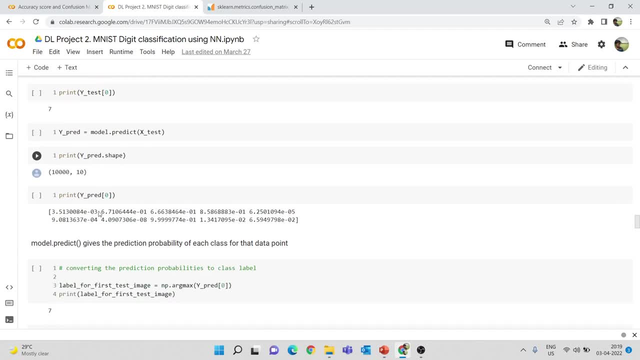 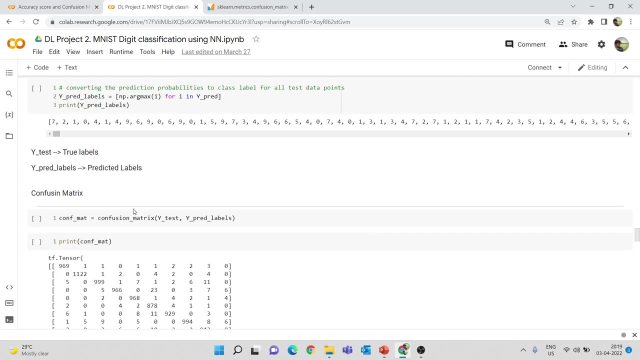 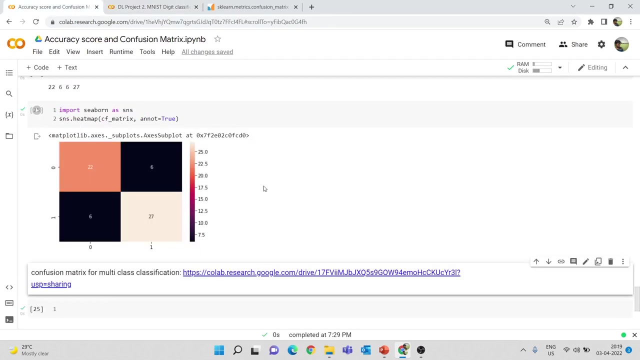 so now let's try to understand how can we build this confusion matrix. so yeah, so this is my confusion matrix. you know function that we are importing, so let me just go to this one. so yeah, so from tensorflowmap, so we don't have to import this from a scale and dot matrix. so this is. 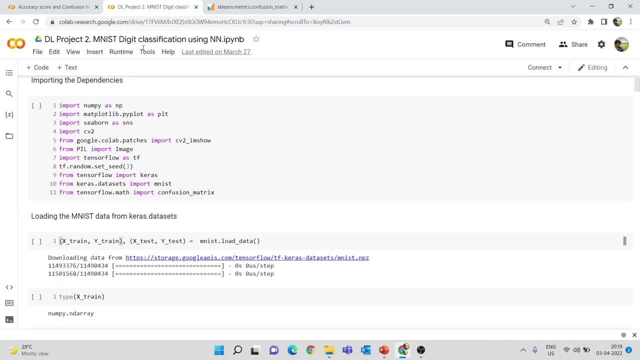 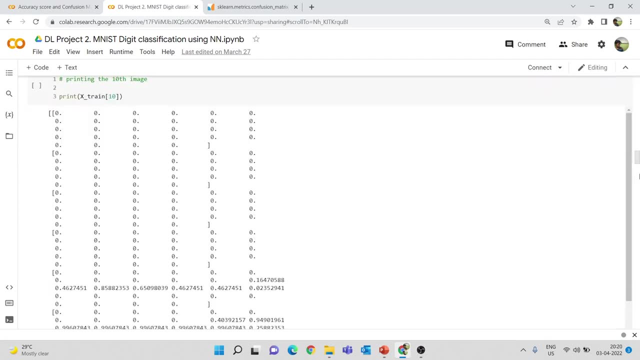 we are importing the confusion matrix from a scalan dot matrix. we also have this function in tensorflow as well, so tensorflowmap has this function called as confusion matrix, but the function is the same. so in both the cases the function is same. in this case, as we are working, 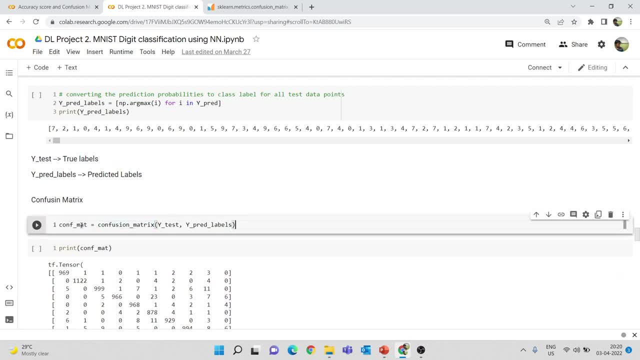 with keras and tensorflow. we are importing the confusion matrix from tensorflow, getting a variable called as confusion. so c o n f mat, which is my confusion matrix, and i'm passing my y test and y pred labels. so y test is my true test data labels and y pred labels is the label. 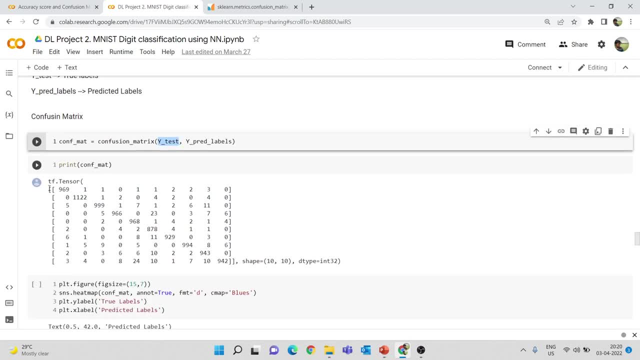 predicted by my model. if i print my confusion matrix, this is the value that i'm getting. so in this case this won't make any sense. and now we can pass this confusion matrix to an eat map in order to understand this better. so here i'm building a eat map, so plt dot figure where i'm. 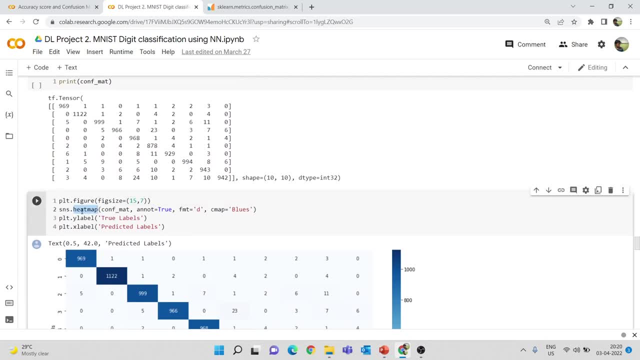 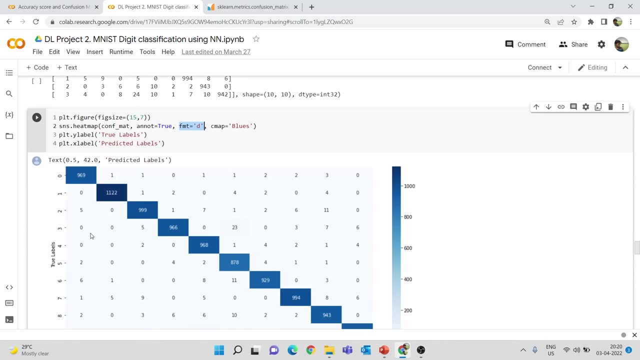 setting the size of this plot. and i'm saying sns dot, eat map. so i'm constructing an eat map with this confusion matrix. i'm just mentioning that annotation is equal to true, so fmt is equal to d means i want all the values in the form of integers. so i don't want any values in floating. 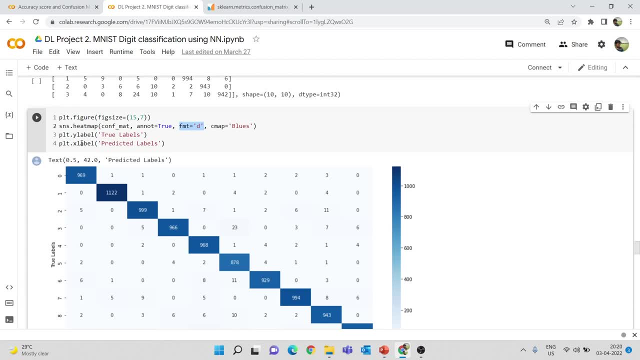 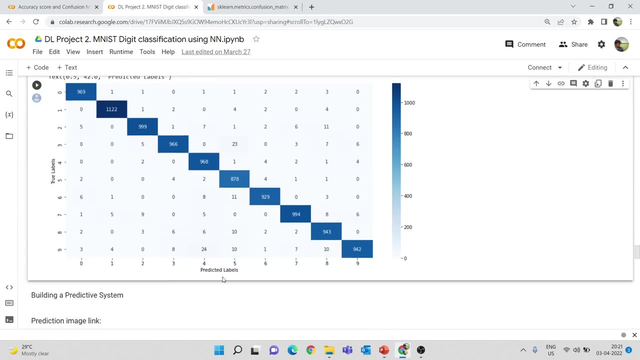 point values, c map lose. so i'm just setting the color of this heat map. so plt- y label and x label. so i'm going to set the true labels as my y axis and predictor labels as my x axis. now let's try to understand how we can infer this. so this is actually the same data. 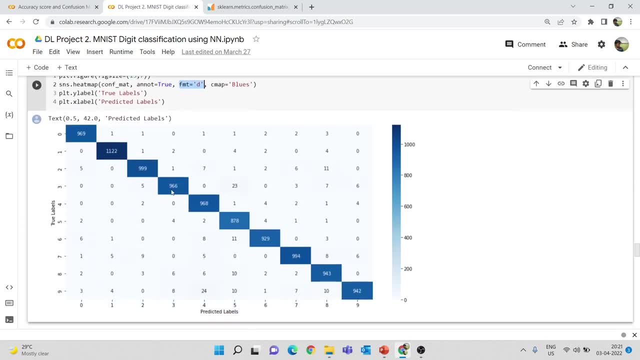 that we have in the previous video. so let's try to understand how we can infer this. so this is actually the same data that we have here. so instead of having this in numerical values, we are constructing an eat map. now let's try to understand. what does this signifies? i told you, 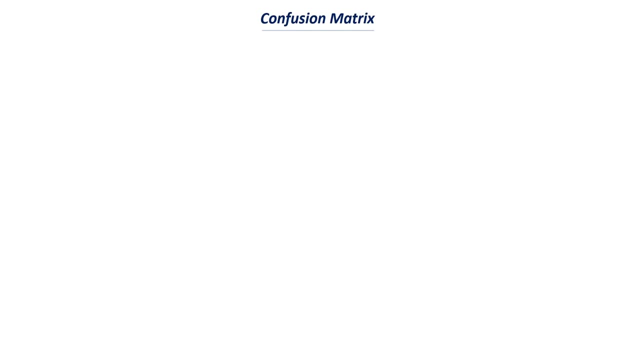 right when the two classes match. so in this case, so we have positive and positive. that means, uh, the predictions are correct predictions. so in this case, we have negative here and negative here. so this is my two predictions. so in this case, uh, positive or negative, so there is a mismatch in. 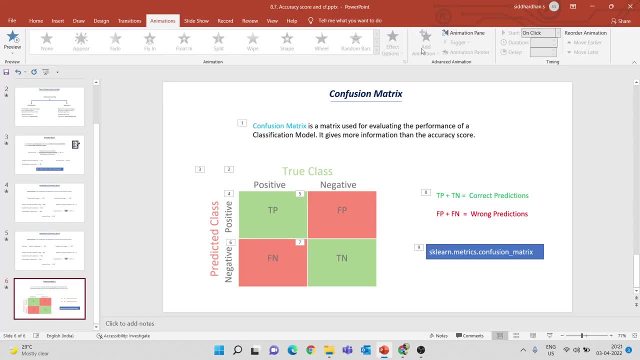 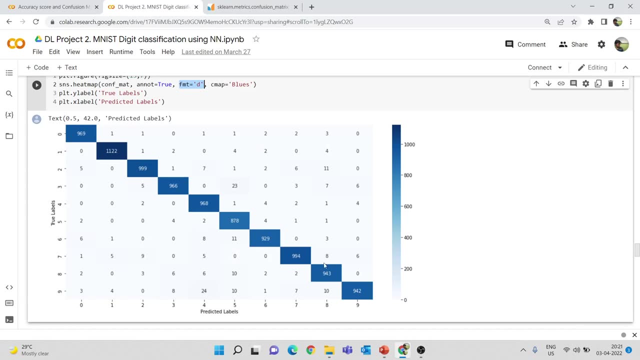 the class in this red color quadrant, in this red color quadrant. so you have to check whether the classes are matching. so this diagonal thing, so all the values in the diagonal, represent my correct prediction. because if you see the corresponding labels here for this first quadrant, uh, the y-axis value is zero. if you 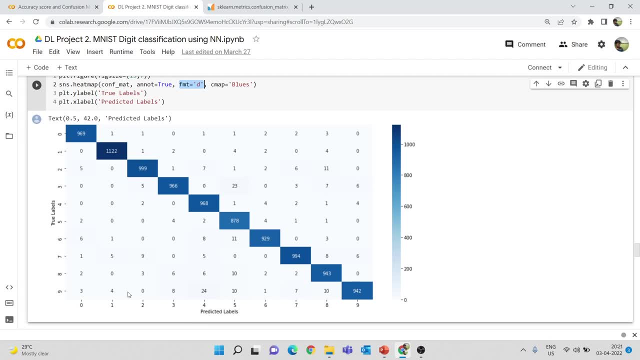 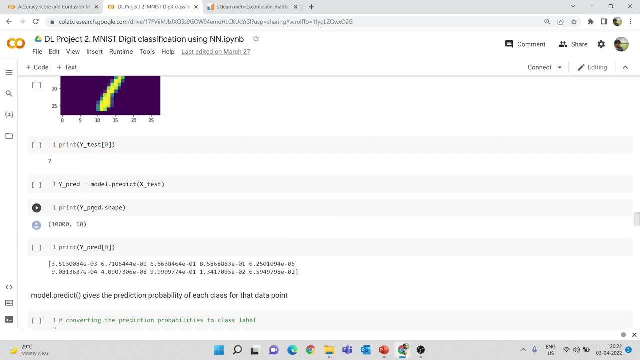 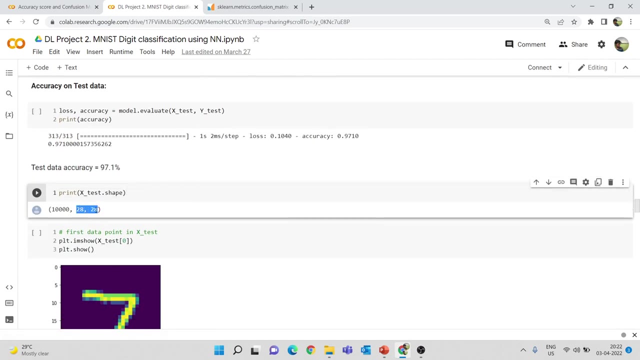 just come to this x-axis label. it is zero. so this is my true label, this is my predicted label. so what does this 969 represent? is, if you go to this y test prediction, so let me go here. so x test dot shape. so this is the pixel size of the image. so it is like at 28.9. 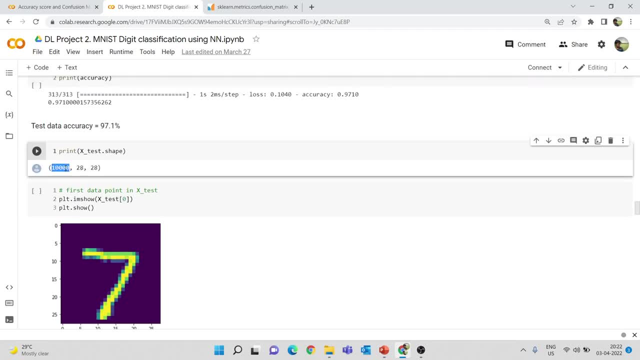 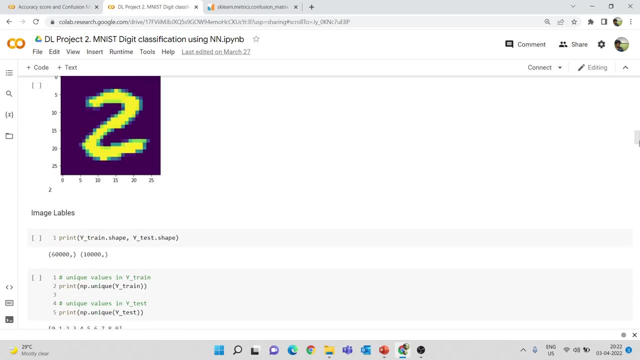 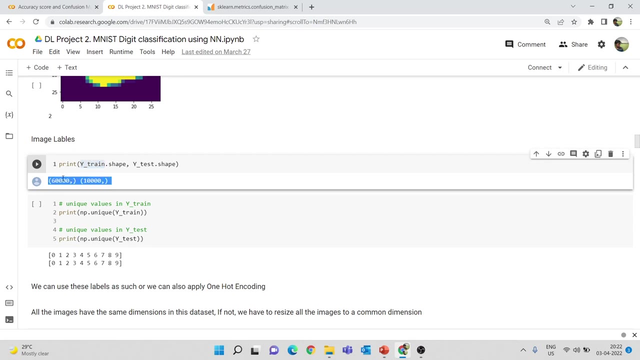 into 28 image and the total number of test data points that we have is 10 000. okay, so, in this case, the training data, let's see, uh, the number of training data that we have here, i think, is 10 000, yeah, yeah, as you can see. so this is the y train ship, y test ship. so, totally, we have sixty thousand. 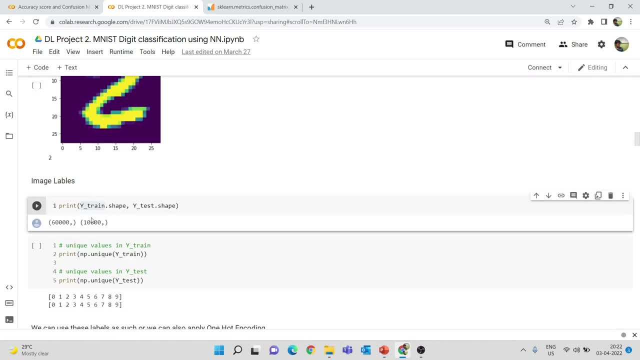 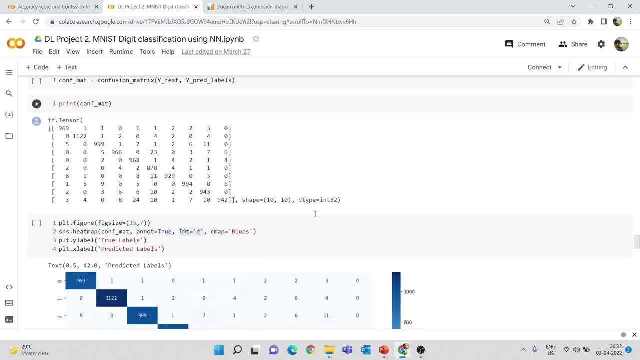 training data images which are like sixty thousand images of numbers and ten, ten thousand, uh, uh, you know, test images. so the uh, so the totally. there are like ten thousand test images and out of those ten thousand test images, nine, sixty nine images have the label zero. that means that image. 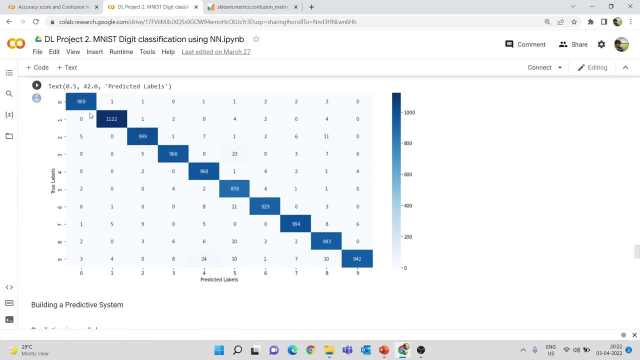 represents zero and uh, this 969 images- has been correctly predicted as zero. so that is what we have here. so you have to see the y-axis label and the x-axis label. consider this as x-axis and consider this as y-axis. so 969 uh images. uh represent zero and those has been predicted correctly as. 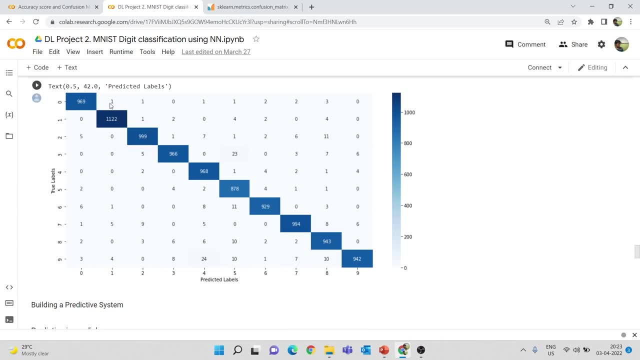 zero. so that is a match of class. if you see the next quadrant value, it is one that means image, and the true label of this image is: zero has been predicted as one. so what does this signifies is, uh, an image that has the image of zero has been predicted as one, and in this case, one again. so in 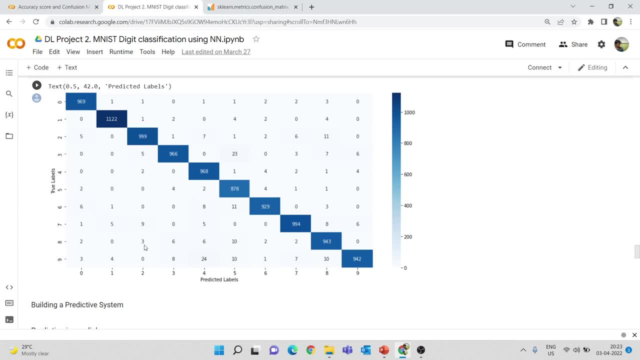 this case, only one image, which is actually zero, has been predicted as two. so that is what these values represent. if you see this, three, so three images which actually represent zero, has been predicted as eight. so this is how you can infer this confusion matrix. so if you see this one one 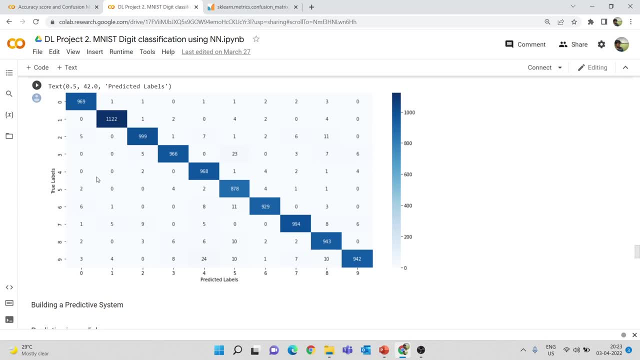 hundred and twenty two values, uh, represent the image one and they have been correctly predicted as one. so, if you see this, four images of one has been predicted as eight and so on. so if you see which, as the highest value, 24. so what does this 24 means is the true label for these 24 images are. 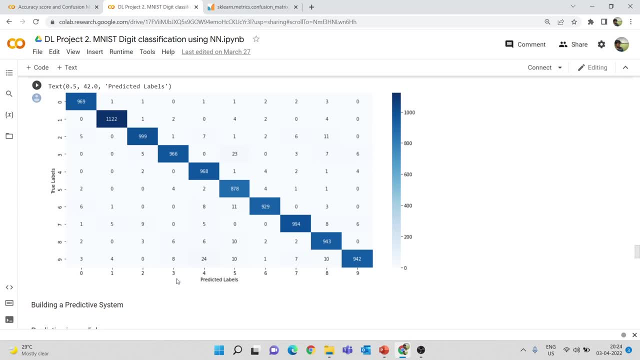 9, but they have been predicted as 4, so you can just understand like 9 and 4 may kind of look similar to the model. as you know, these are like handwritten images, so these 24 images has been uh 4, so 9, like 24 images of 9, has been predicted as 4.. so, whereas if you consider this one, so there. 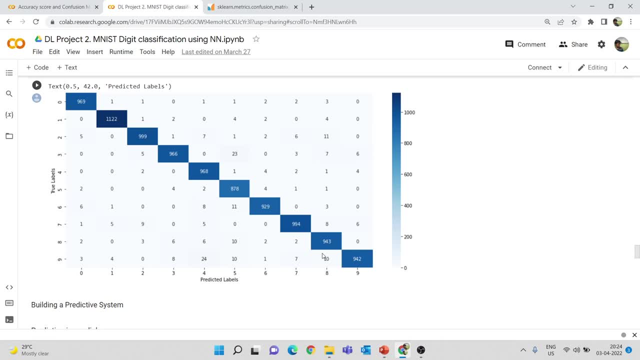 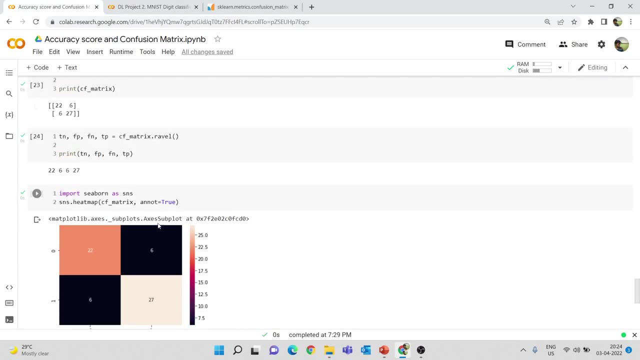 is 9 here and there is 9 here, so that is match of class. so this is how you can, uh, you know, infer a confusion matrix in the case of a multi-class classification problem. and it is always better to load this confusion matrix into an eat map to understand it better. so if there is a match, 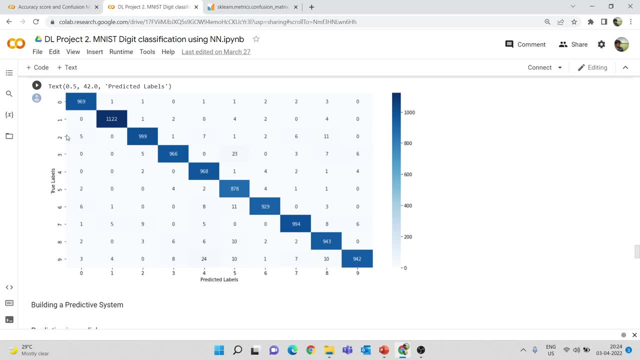 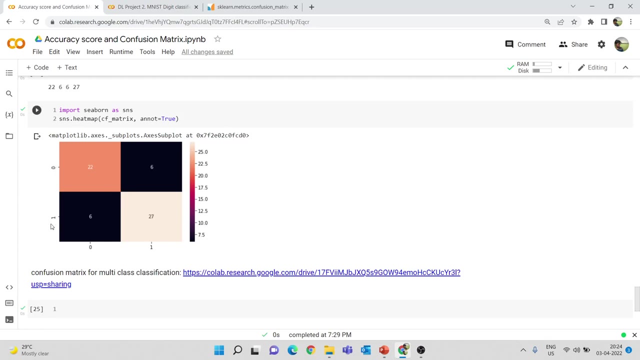 of class, then in that case it represent- uh, you know- correct prediction. if there is like mismatch, it represents wrong prediction. or the other thing that you can understand is: this diagonal represents my correct prediction, all the other uh values represent my wrong prediction. so here also, this diagonal represent my correct prediction because we have match of class 0 and 0, 1 and 1, so 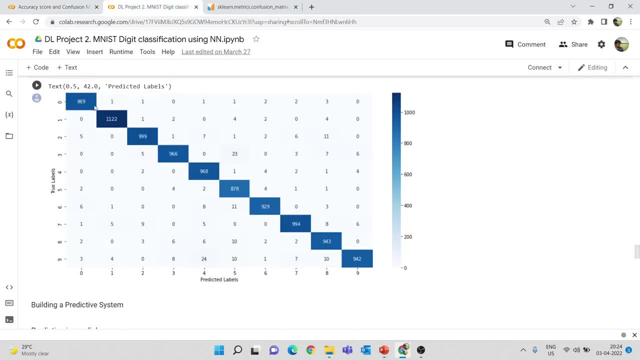 for this. so, similarly, we have the 0 and 0 here, 1 and 1 here, so this diagonal represent my correct prediction. so this is how, uh, you know, we kind of uh- use this confusion matrix in order to understand, like, uh, we kind of like understand- the performance of the model better, whereas in 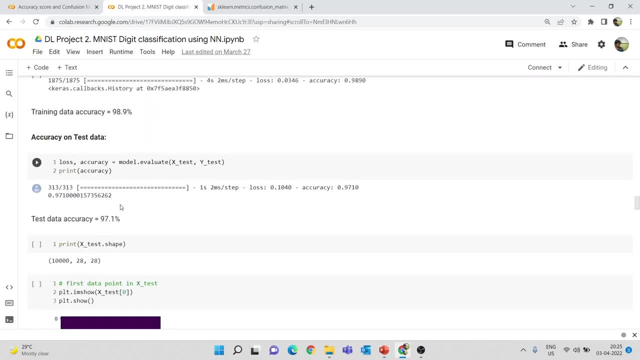 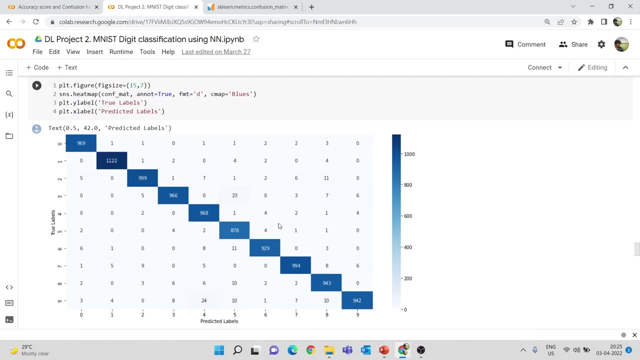 the case of accuracy score, it will just tell you that. so, out of untread images, 97 images will be predicted correctly, and for thousand images, 970 images will be predicted correctly. so this is what this accuracy score means, whereas if you build this confusion matrix, it will tell you what images are being being predicted as what.